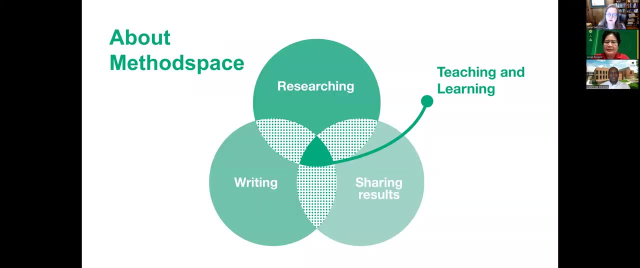 But before we get started, if you are new to Method Space, this is a web community hosted by SAGE Publishing and we're interested in everything to do with research, design, planning, conducting, analyzing, writing about what we find and sharing results in all different 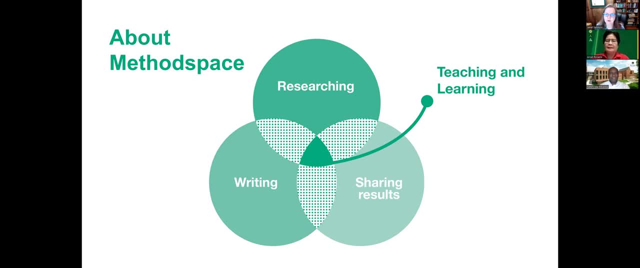 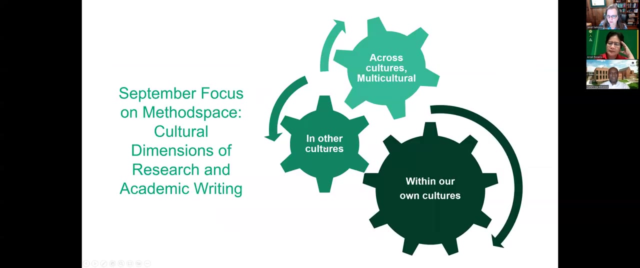 kinds of ways And, as you can see, at the heart of this diagram we have teaching and learning, because we think that whether you are a brand new researcher or a very experienced researcher, we all have something to learn. And this month we're kicking off with this interview and we're going to be focusing on cultural dimensions of research and academic writing, thinking about kind of considerations for research within our own cultures when we venture into other cultures. 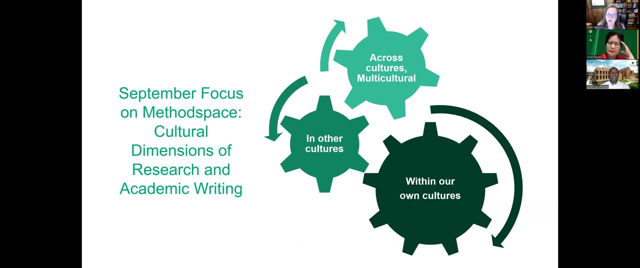 and when we do research across cultures with a variety of research participants and collaborative partners. So I'm delighted to have both of you here to help us think about some of these questions this month. Why don't you just start by briefly introducing yourselves, Arceli? 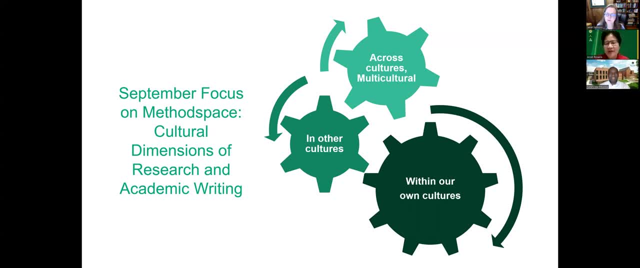 All right. so I'm Arceli Rosario Safari and I met when we were teaching at the Adventist International Institute of Advanced Studies, and it was during this time that we worked together that he invited me to be part of what he was trying to conceive as the Asian Qualitative Research Association. 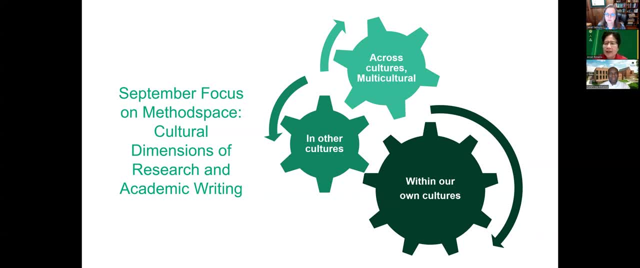 I gladly joined him, and there's another one A colleague, Sonia Fokufoka, and the three of us sort of like initiated this association of qualitative researchers. We started in 2015,, and our aim was to empower qualitative researchers, So I was part of that work. This association grew big until 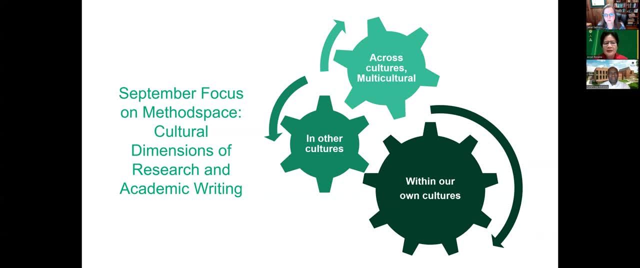 we thought that it was the right time. after conducting many trainings on qualitative research, we thought that it was time for us to write books. So that was a big part of who I am. I became a qualitative researcher and got involved in the lives of many people, So I stayed at that school for 10 years. 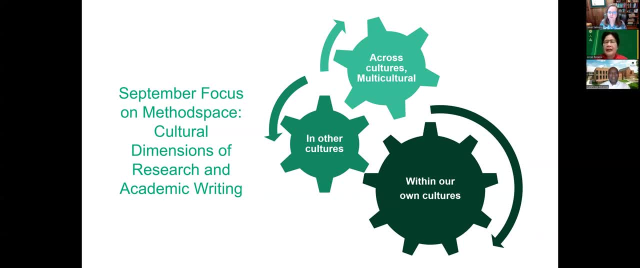 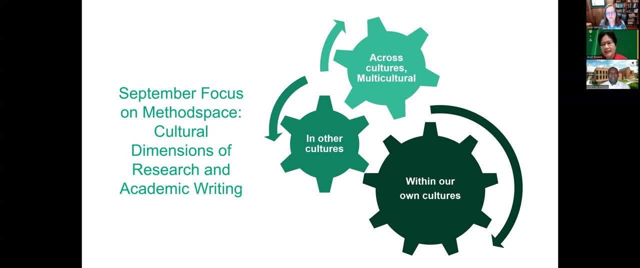 where I served as its president. where I served as its president. Thank you, Safari. I'm Safari Ombaleca and I approve of everything that Arcelia said. I'm Safari Ombaleca and I approve of everything that Arcelia said. 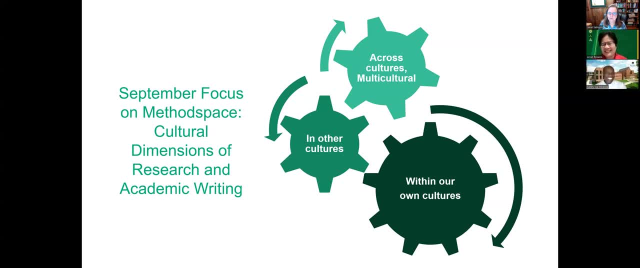 I'm Safari Ombaleca and I approve of everything that Arcelia said. We have worked together since I think it was in 2010.. We have worked together since I think it was in 2012.. We have been colleagues and friends and we really think alike as far as qualitative research is concerned. 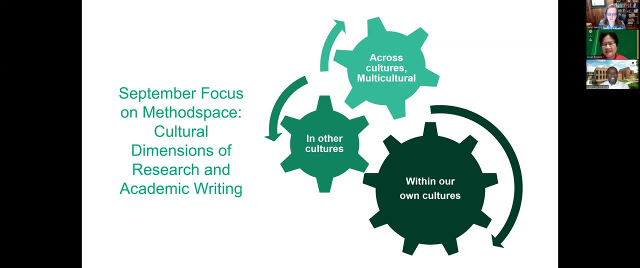 We have been colleagues and friends and we really think alike as far as qualitative research is concerned. We have been colleagues and friends and we really think alike as far as qualitative research is concerned, And I'm currently serving as an associate professor of leadership in higher education at Bethel University. 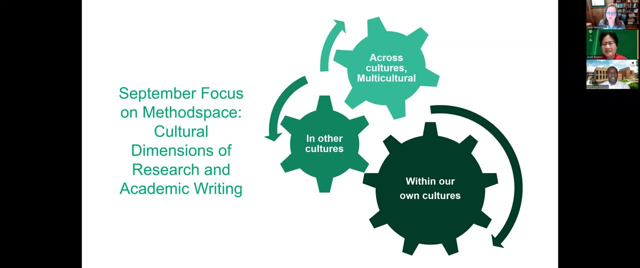 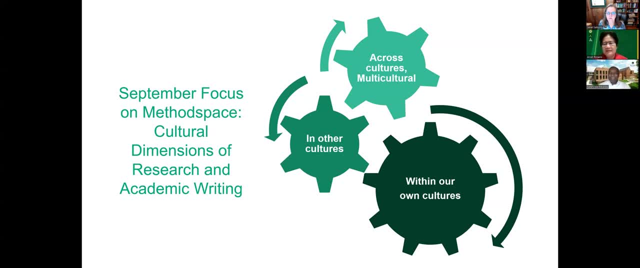 And I'm currently serving as an associate professor of leadership in higher education at Bethel University. And I'm currently serving as an associate professor of leadership in higher education at Bethel University And here I teach research classes and mainly qualitative research classes, and I'm a. 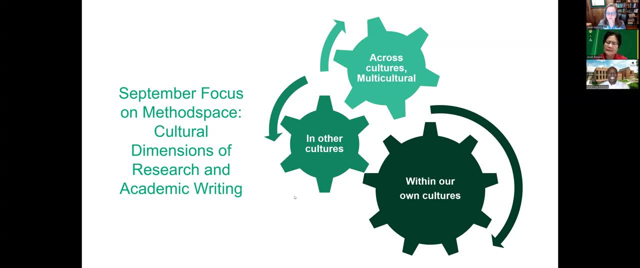 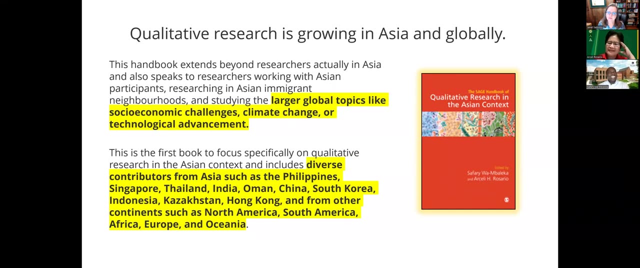 methodologist on dissertations. This is only the doctoral program of educational leadership here at Bethel University, And I'm just so excited that this dream that we had about maybe back in 2018, actually, we started thinking about this a number of years ago, but we kind of kept it on the 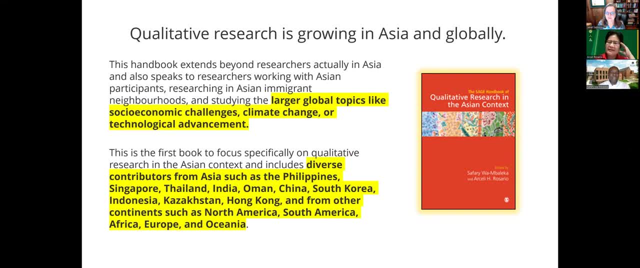 background, but it has become a reality in 2022.. We now have the quality, the sage handbook of qualitative research in the Asian context And I'm just excited that we have this resource and that will be a great blessing to many people around the world. 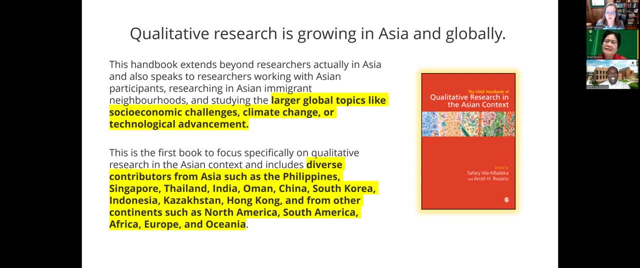 So could you start by? you know we can see here, you know on the screen, you know where. you know some of your contributing Authors are from um. could you just talk a little bit about some of the cultural contexts? 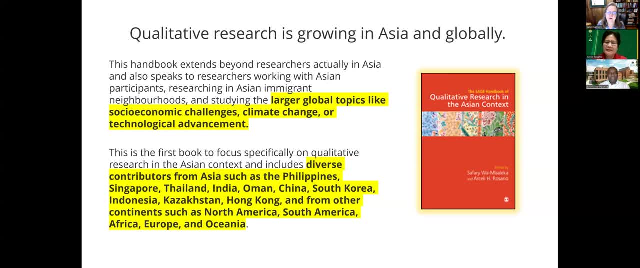 and, oh you know, co commonalities and differences across these cultures. So, or Sally, why don't you start? Yes? So when we conceptualize the book and specifically who the authors would be, our first consideration was, of course, um, people. 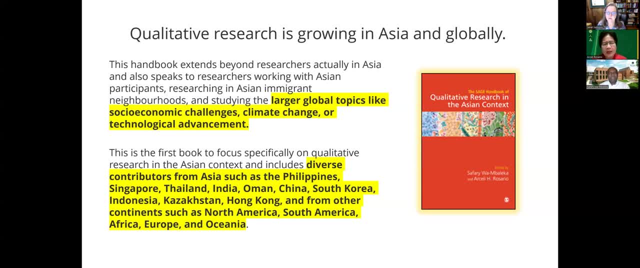 Authors coming from Asia. So we thought of: okay, so who are the experts in qualitative research in Asia? We started looking at those very near us, meaning faculty and alumni of, uh uh, the Adventist international Institute of qualitative research, because that was where. 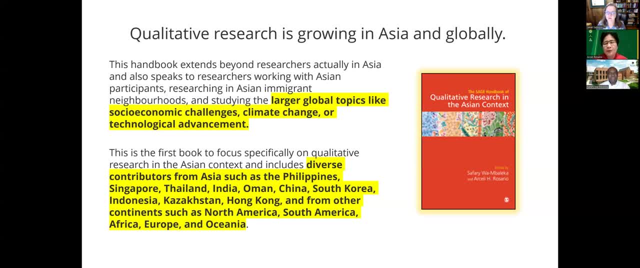 Accra, the Asian qualitative research association was born and it was there where we heavily invested our time in terms of training, developing resource speakers in these trainings. So we we focused on these people and, fortunately, people at the Adventist international Institute of advanced studies come from different places in the world. 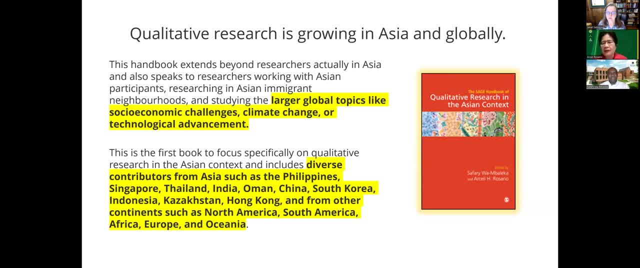 Uh, our students and faculty represent around like 80 countries. So, uh, we got them, I think, because, uh, they're expert in qualitative research. also because, um, yeah, we know them and it was easy to reach them and they, they had engaged with us in many ways, in many. 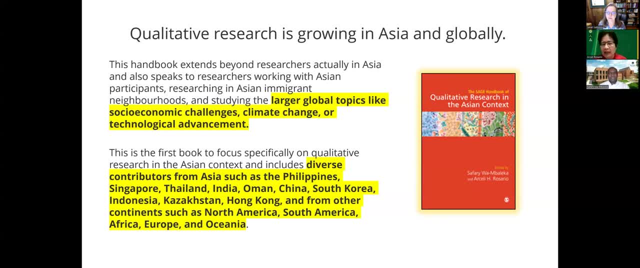 occasions. So we thought of them and and, uh, some of them, actually At the time when we conceptualize the book, had already moved to their country. So, for example, uh, we had a faculty alumni who, um, already 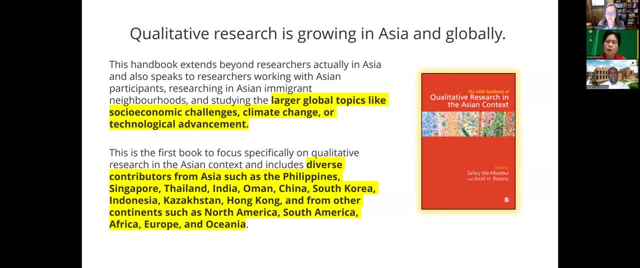 Moved, went back to Argentina, to Romania and other places. but we were also intentional in thinking: who are the experts in qualitative research in Asia? So we reached out to uh experts that we have uh connected with Uh. 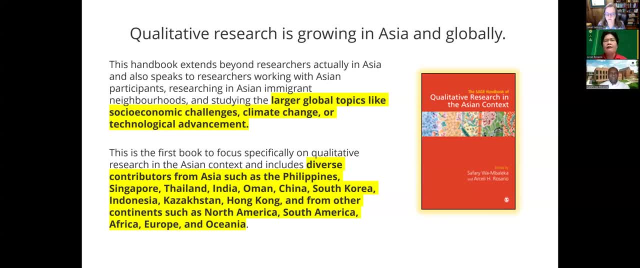 In fact We had one coming from Hong Kong, from in Kazakhstan as well in Vietnam and, of course, in the Philippines, in other places in Asia, And we also identified qualitative researchers from other countries, for example the United States, who had been conducting qualitative research in Asia. 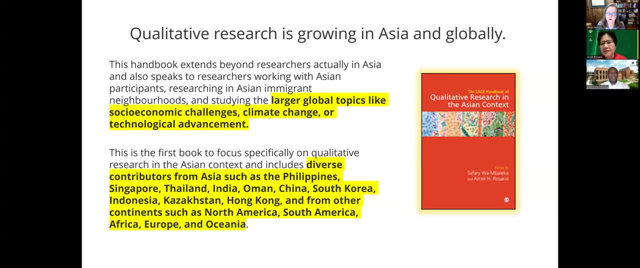 Safaree, what would you like to add? Yeah, if I may go to the question of commonality, I think you had kind of mentioned that- what is really common in the cultural settings in Asia For me as a foreigner to the Asian context? I worked there for eight years, specifically in the Philippines. 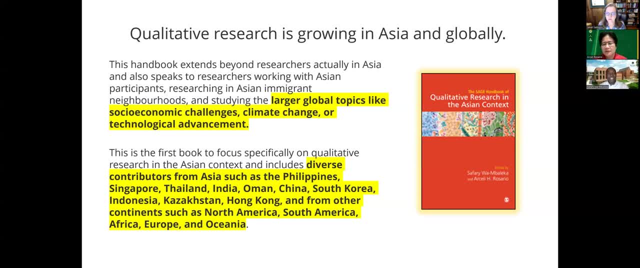 but I got to travel To different parts of Asia, Southeast Asia specifically. There were things that were common- and you see these going through the whole handbook- and that is the concept of respect, for example. Respect may be expressed differently in different parts of Asia, but the concept of respect is very strong in Asia. 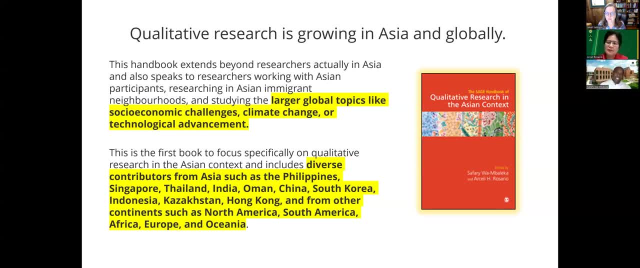 And I think this is common to Eastern cultures, including Africa As well- that people who are in position, people who are in the power, people who are older than one is. they deserve respect And they expect it is expected when we are communicating with them. 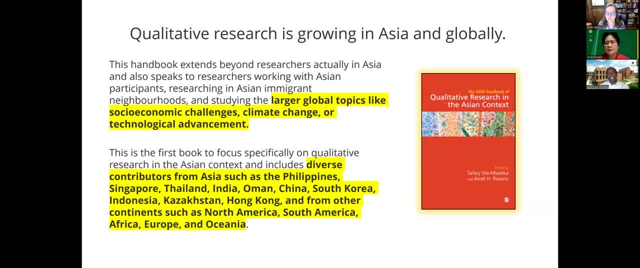 It is something that has to be taken into consideration. The other commonality in Asia: in most parts of Asia, probably other than Southern Europe and North Korea and maybe Japan, most countries in Asia have several languages. So when we are conducting qualitative research in Asia, we have to make sure that we are going to deal with a 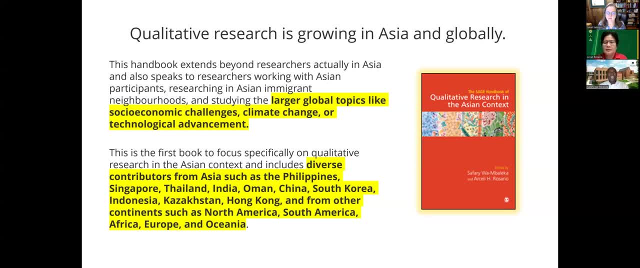 different linguistic variation, And not only because everybody is from the Philippines. um, we cannot take it for granted that all the Filipinos will address things the same way, because, just to take the Philippines alone has 82 languages, And those 82 languages for those. 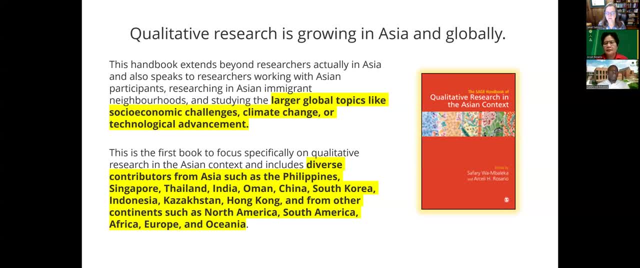 who study languages, we know that language and culture go hand in hand. That means those are 82 subcultures that you have in the Philippines. Indonesia has more than 600 languages. That means Indonesia has more than 600 languages And that means that Indonesia has more than 600 languages. 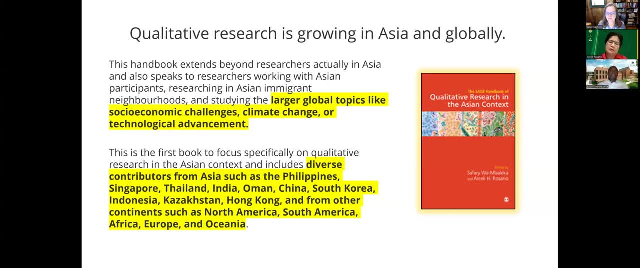 600 subcultures. So, in addition to having one thing we can call a national identity, cultural identity, you still have some subcultures that when we are conducting research there. even personally, as a foreigner, when I was conducting research in the Philippines- 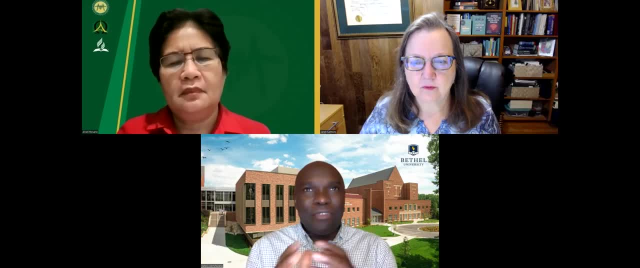 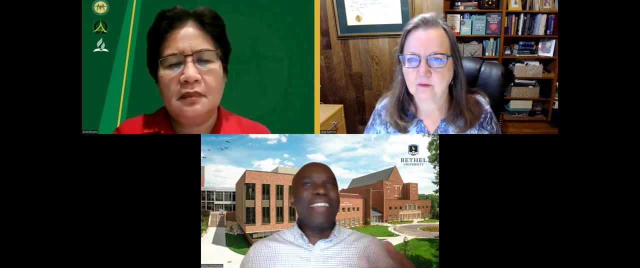 I had to know these differences, to be aware- probably not know everything, but to be aware that, hey, people in the North may react to certain things differently from the people in the South of the Philippines, And so language respect and many other details that we discuss in the handbook. 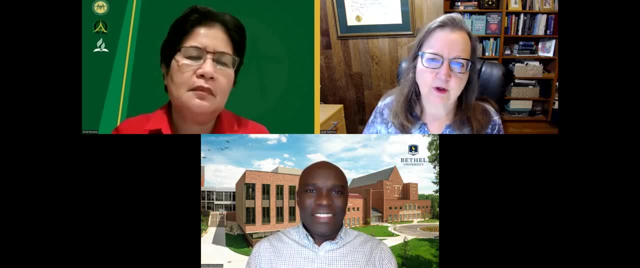 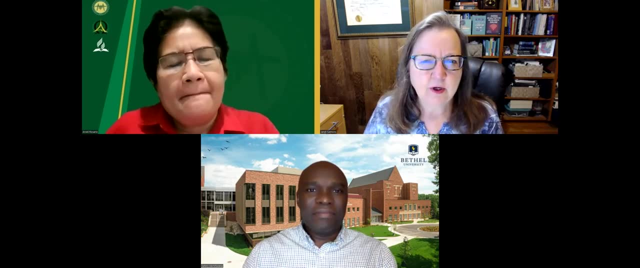 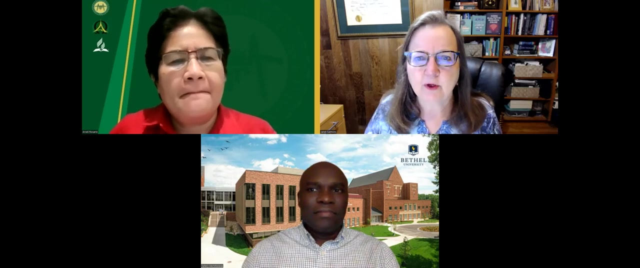 So well, I mean, it's interesting, you know that you, you know- highlight that point because I think you know for qualitative researchers, where you know there certainly are qualitative researchers who work with, even, you know, big data, with BigQual, but you know the kind of 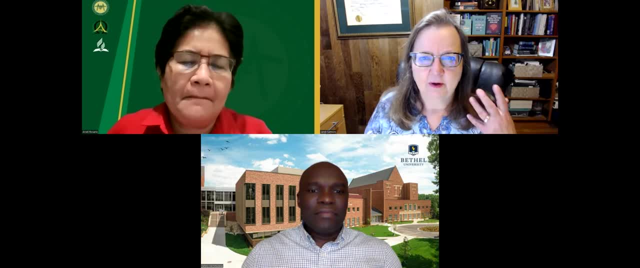 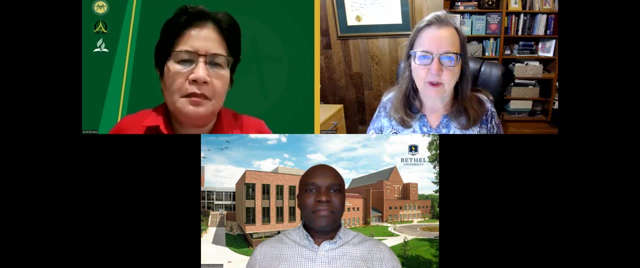 characteristic of qualitative research of being more, you know, people-oriented, and you know the relationship that some of the kinds of things that you bring up would be really important for qualitative researchers to understand. So you know, I wanted to just ask. 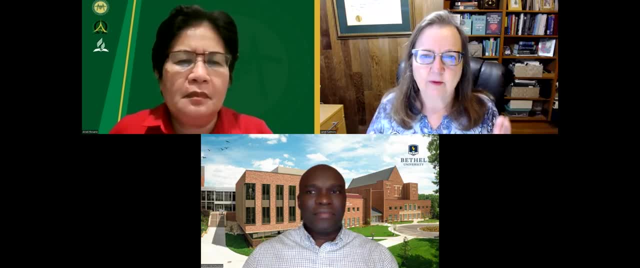 you know what you know with the, with the work that you've done with the Asian Qualitative Research Association and with the, with the evolution of this book. you know why are qualitative researchers. you know who are qualitative researchers, who are qualitative. 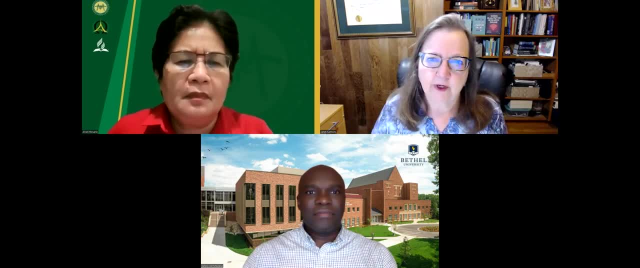 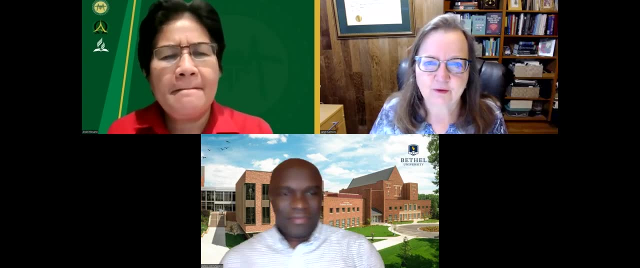 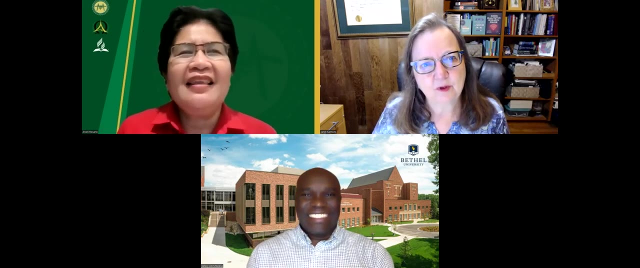 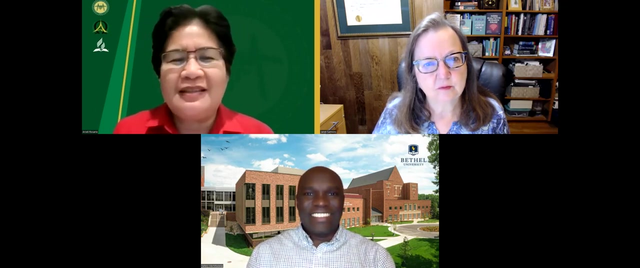 research methods. appealing to Asian researchers: What is it that they like about qualitative methods versus other ways of doing research? Let's hear from Marcelle first. Okay, so let me begin. I think there are some reasons why Asians are attracted to qualitative research. Let me first speak in my own perspective. So 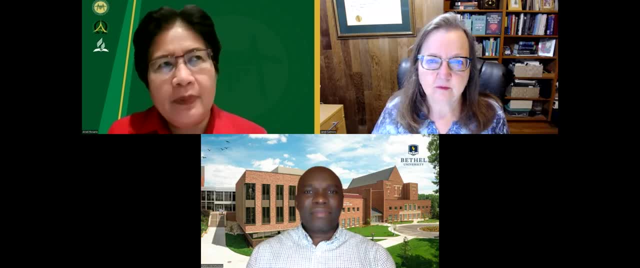 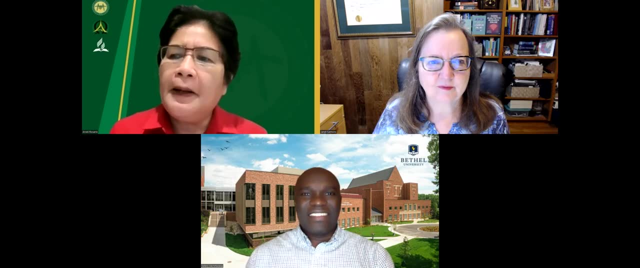 you see, I think as a people, we love to talk and we love to share matters that are private to us. It's natural for us to, even to people who may not be very close to us. it's it's acceptable, For. 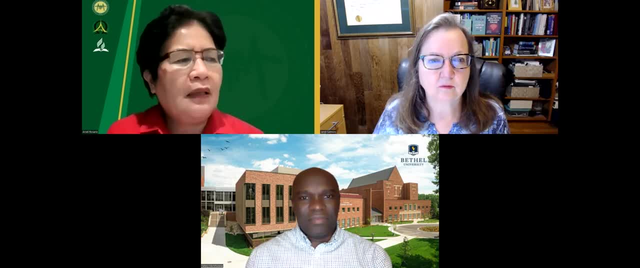 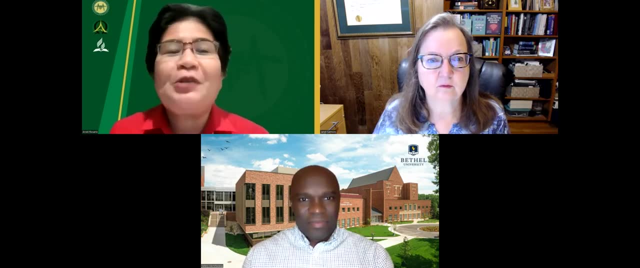 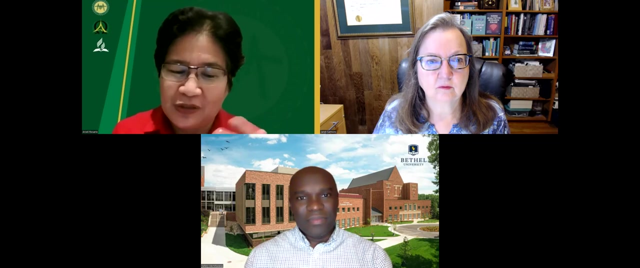 one to talk of feelings. shall we say feelings or how we look at things, or exactly our stories? Mm, hmm, It's easy, it's like natural for us to talk, share with each other, with friends, And even with not so close friends, even with people who just come to the community. 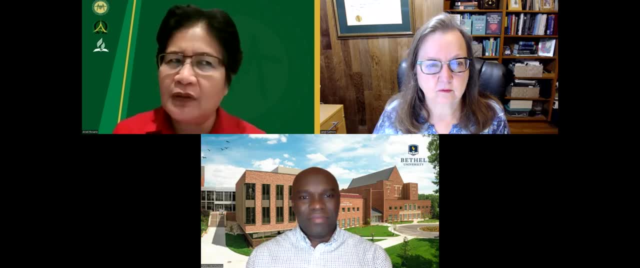 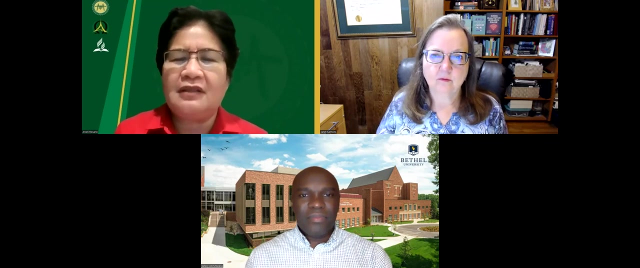 and ask us to share stories or praise them. it's not acceptable For one to talk of feelings. ask us to share stories. that is not a problem at all. so when I did my master's and when I did my dissertation, I I adopted the qualitative, I chose qualitative research because I felt it's a natural. 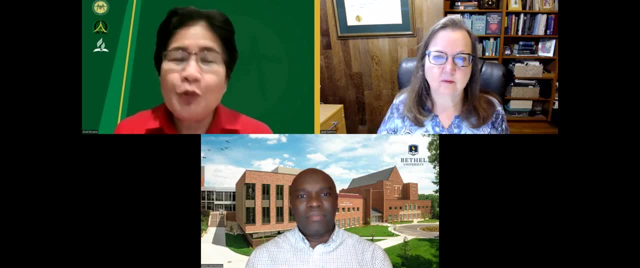 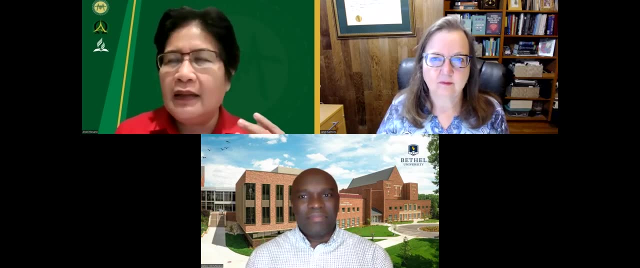 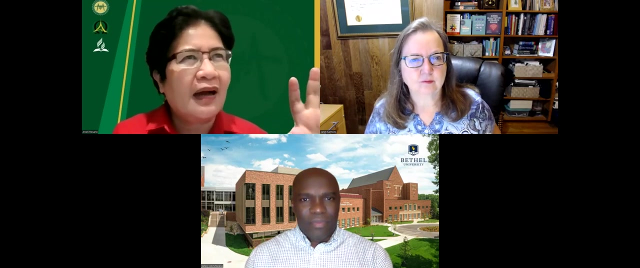 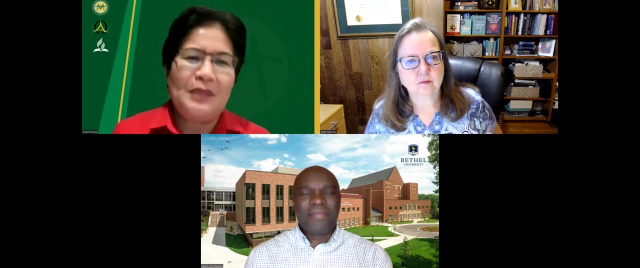 thing for me to do, that as a researcher, to talk to people, it's. it's very fulfilling for me to go to uh. so for my master's I had to uh retrieve oral literature in uh uh. you know, in a village I had not met these people, but it was easy for me to do that. so as a researcher it's not a problem. 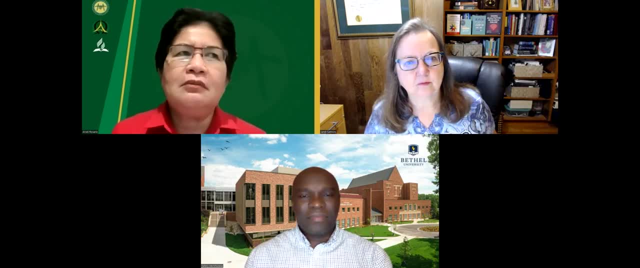 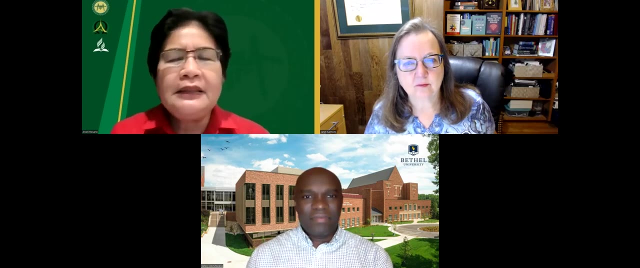 at all, and when I did my dissertation, I did with women university uh leaders, and those were women I had not met in my life and they were coming from, I would say, very respectable uh place and I did not even doubt for a second that they would not give me time, so it's like I was looking at my perspective. 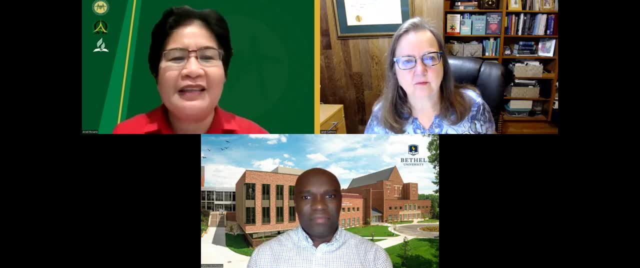 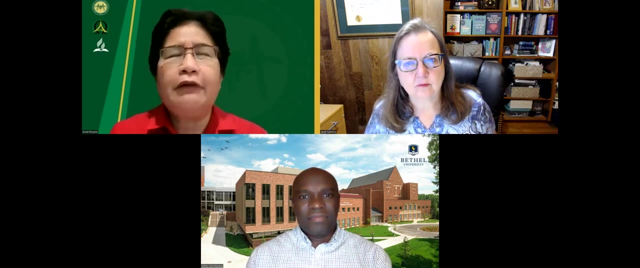 I like to talk to people and I did not doubt that they would also love to talk to me, and it proved that way. so, um, I'm speaking specifically as a Filipino, but I think, uh, it's true to- I don't know, maybe not all, I don't know- Safari. I haven't uh traveled really or talked to people. 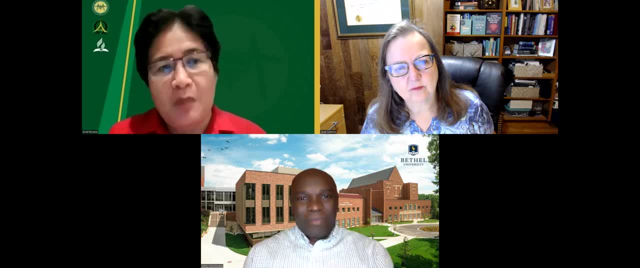 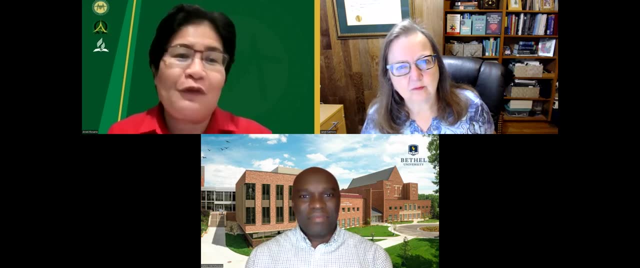 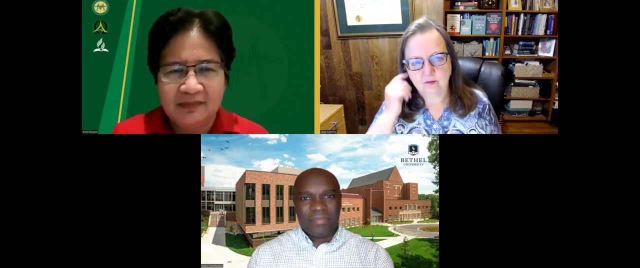 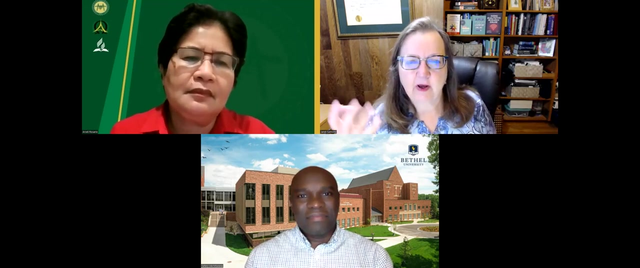 in all of these Asian countries, but I think to most we like to share our stories and it's like, uh, it's very fulfilling for us to do that. so it's appealing because in qualitative research you get to do that. research now becomes a very exciting venture. yes, so, um, given, given that you know, kind of tapping into the, the oral culture and the. 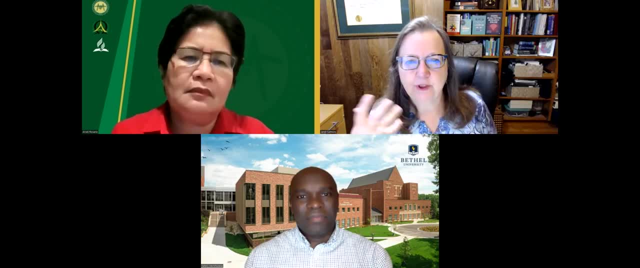 kind of storytelling and and personal sharing uh. so you know what kinds of methods uh do researchers favor. so it sounds like perhaps uh interviews, uh focus groups or group interviews. you know what kind, what kinds of data do you use to do that and what kind of data do you use to? 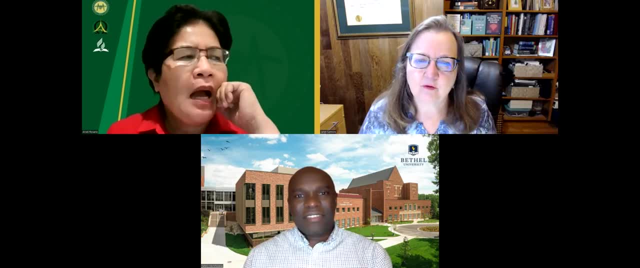 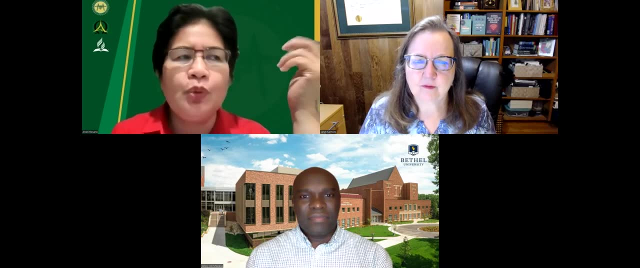 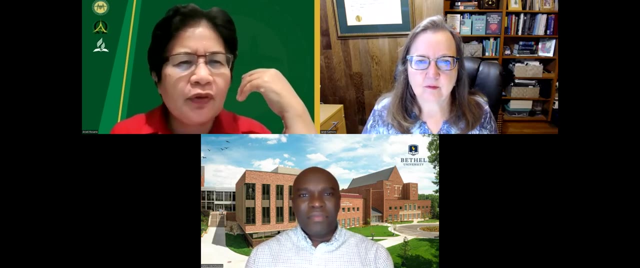 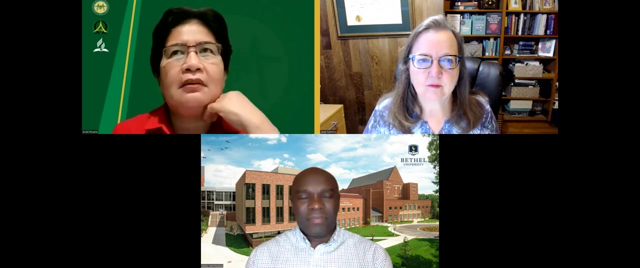 data collection methods seem popular. yeah, I would say, like the in-depth interview, the one-on-one interview, which is very intimate and you really get to share um your inner thoughts, your deep feelings, this come, this method, uh, data collection method comes uh natural for for us, for us. 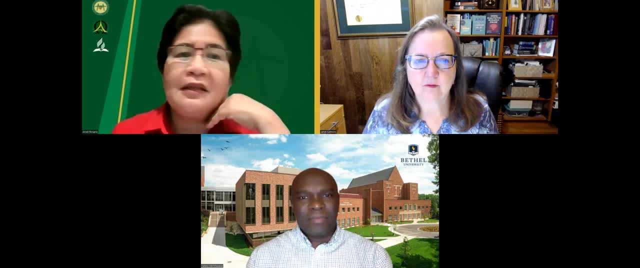 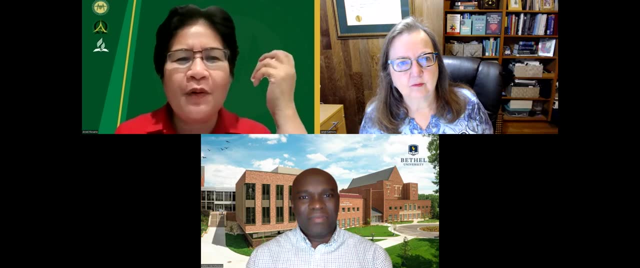 that's all Behrooz has mentioned so far about. the new challenge for us is how to and how to communicate, and so I think it's fascinating to just to kind of follow that you know first issue and then talk about the challenges that we need to address, because it's also a very different. 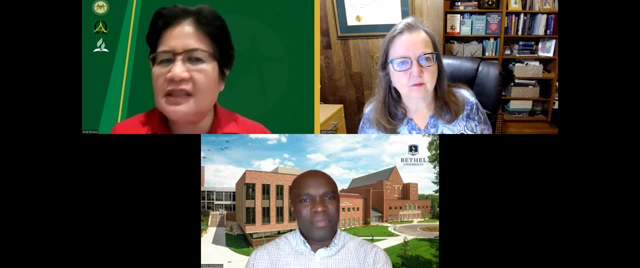 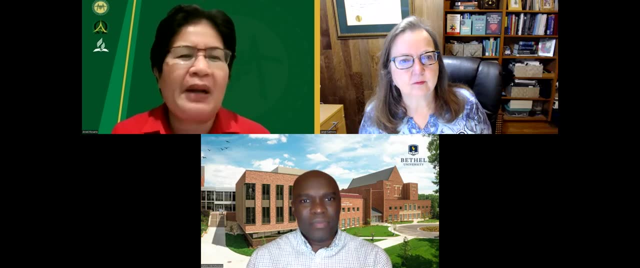 question because it's a very different piece, um, and it's also a very different question because that's when you look at the application that you have, but for us is very different and it's very different. you know, you, you have to understand the context, you have to understand the. 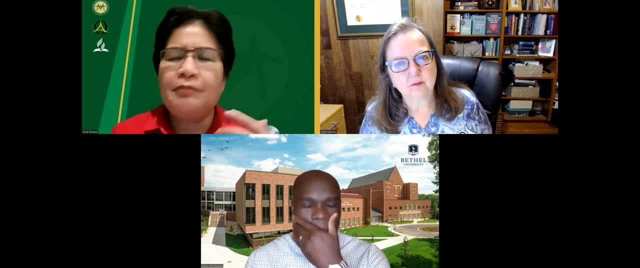 context and you have to really get it through the kids who you know you have to. you have to trust the kids who are in charge in the village and you have to be sure that they are doing that together. when that's facilitated, people come and. uh, even if they meet people for the first time, they are. 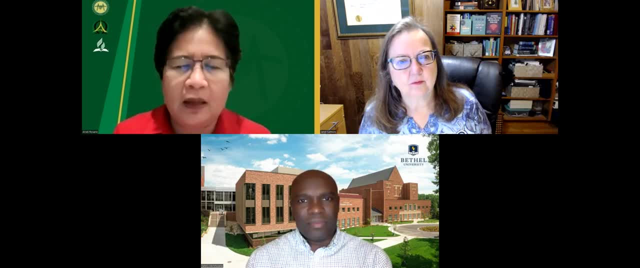 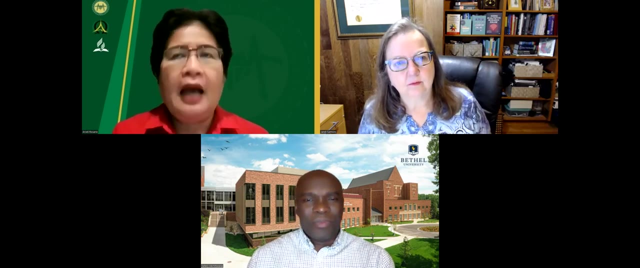 not shy, so host group is is good as well. one methodology, one methodology that i have used and earned some kind of success is photo voice, which is intensive and highly engaging, demanding in terms of time, but uh with. usually i do this with a group, of course, because it's uh, it needs several. 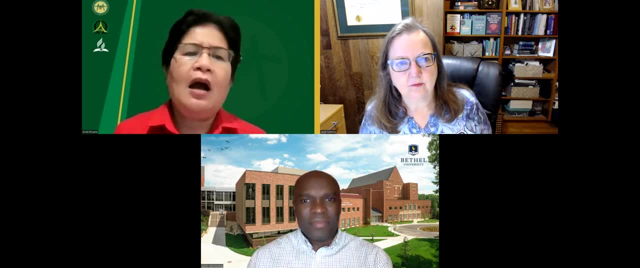 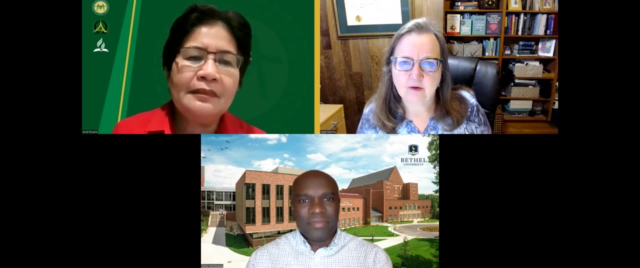 people to do it. so far we have had success. our participants come and we have high- uh, i mean like- retention of participants. anything you'd like to add? yes, anything you would like to add safari? what kind of method for you? yes, i would like to add safari. 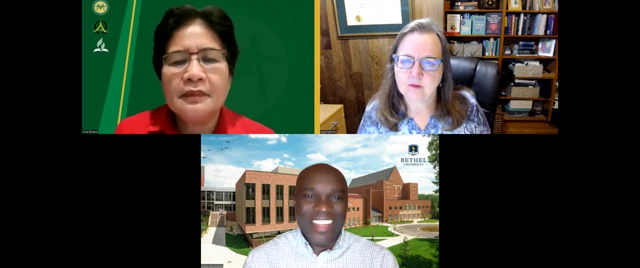 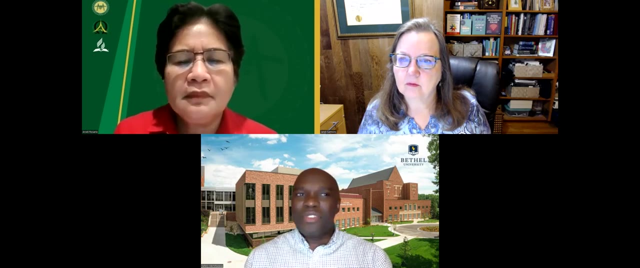 i think. i think this is where we complement each other. to take an outsider's perspective of asia: um. for me, meeting and interacting with asians from different parts of the continent, i classify asia into two categories. um. one category is exactly what arsene has said, which is represented. 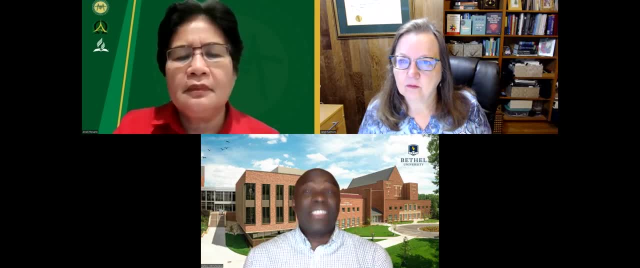 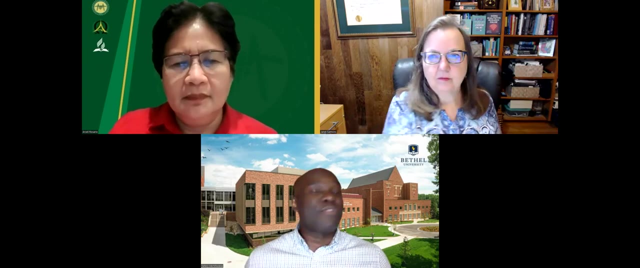 from my experience, represented by the philippines, indonesia and maybe india, where you beat people, within five minutes you have become friends. they even share a lot of information with you. it's like they trust you. i mean, if, if you show that you're trustworthy, within five minutes you can definitely get a lot of information, personal information, and you are asked also. 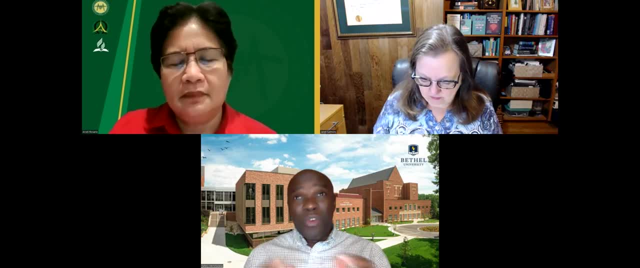 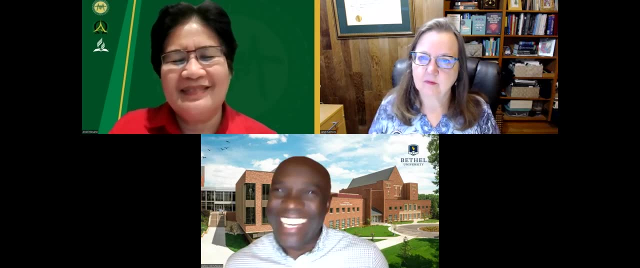 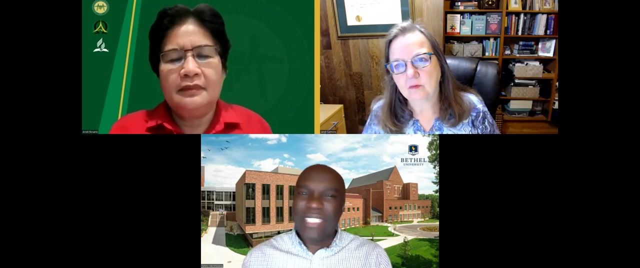 to share a lot of information, personal information. so, with these specific countries, uh, it's only now that it came. it came to me. actually, as i said you were sharing, it never crossed my mind in the past. um to in these specific countries, conducting qualitative research is, i think it's a lot. 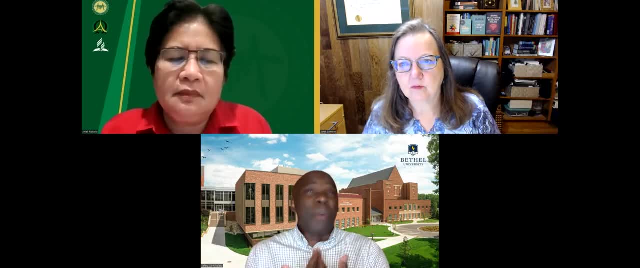 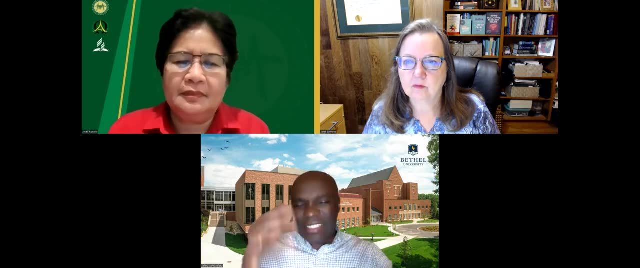 easier because people are willing to share of themselves. it's, it's part of their um, being nice, being kind, being wonderful to other people. i think that's the mindset of what is happening there. then you have on the other side, you have countries. i would say um, i would say it's. 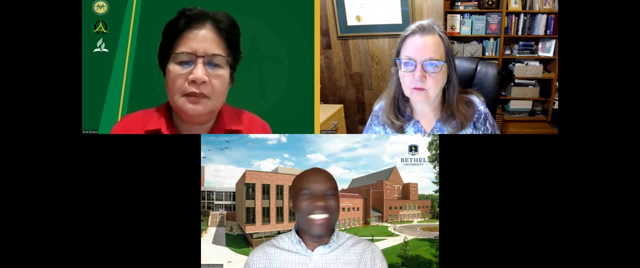 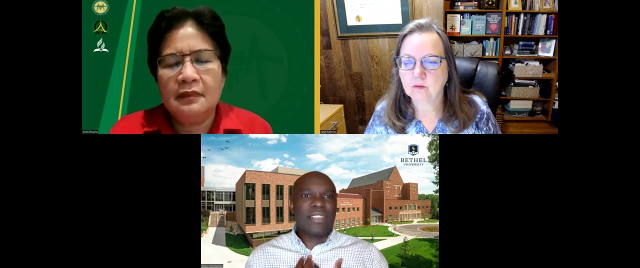 maybe predominantly buddhist countries. i'm looking at thailand, i'm looking at myanmar, i'm looking at uh um uh, maybe others outside of buddhist countries like china, japan, south korea. people are closed. i mean, you can initiate conversation, but to sustain conversation will take some time, unless it's you're talking to people who have traveled a lot. 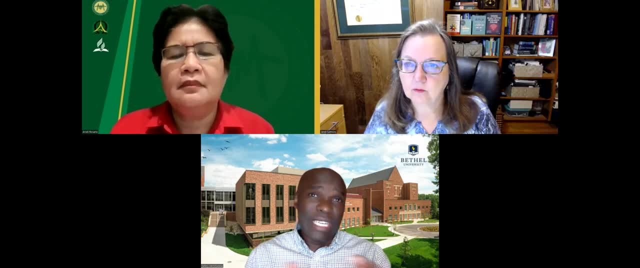 then that is different. but if it is people who have not really left their country, they may not be too much open to foreigners. and so i want to believe for a foreigner who's trying to conduct research when it is research in those countries, it will take some time to build. 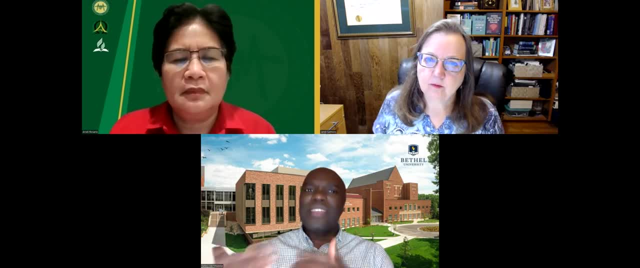 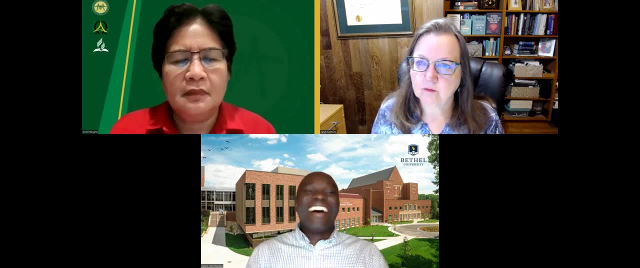 um, trust the trust so that you can conduct research, and so, um, that is, uh what i have seen as an outsider. uh, but exactly what our city said is true. with my experience in the philippines, i conducted and published a lot of research in the philippines. that's exactly what it was within. 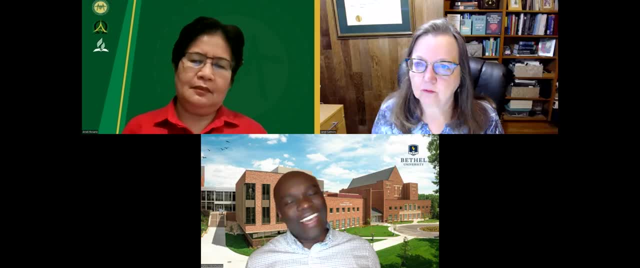 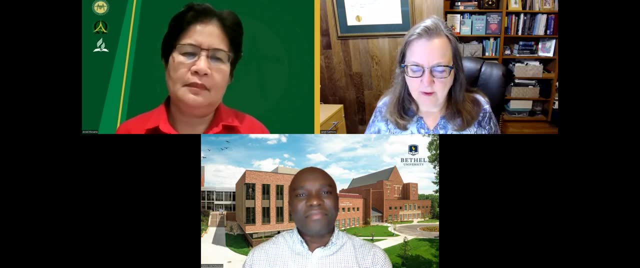 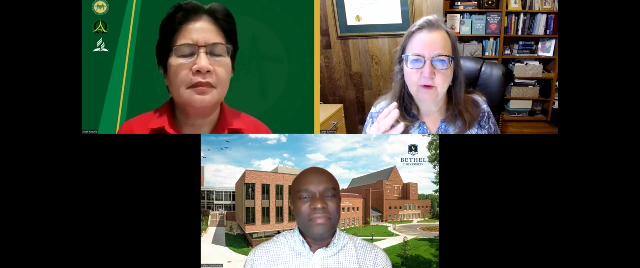 five minutes. i knew a lot of information from anybody i i talked with, because they're willing to share. so, um, you know thinking about uh, you know not only uh, you know the, you know the people who who have studied with you and have now, you know, gone back and they're, you know, you know, back into 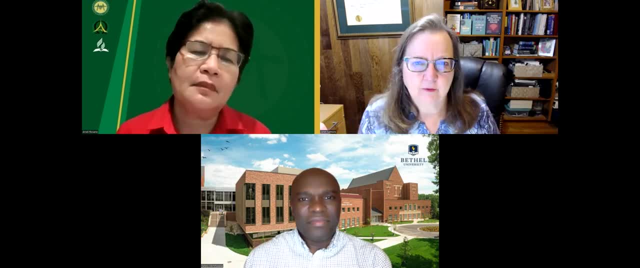 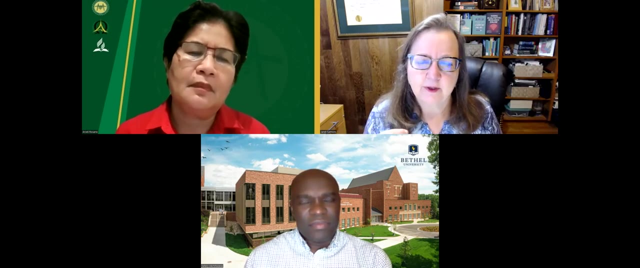 their own countries and you know people who might be um using this book. you know how do you think this will be beneficial to asian researchers who are deepening their skills, you know to conduct research, and and how do you think it will benefit, uh, non-asian readers? 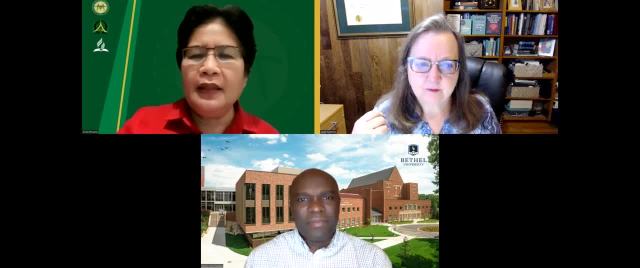 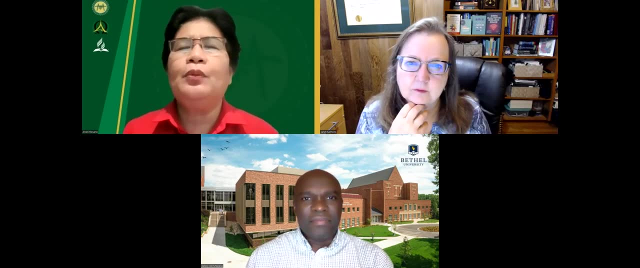 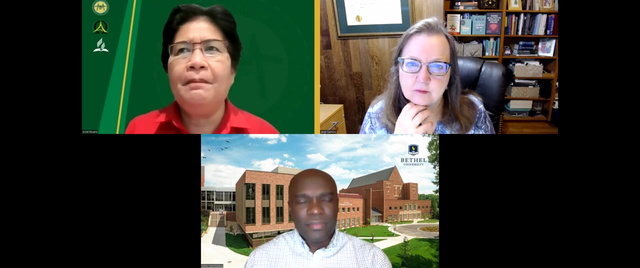 okay, let me start with that. uh, i think i can focus on: uh, how can the book be beneficial to asian researchers and how can the book be beneficial to non-asian researchers? uh, firstly, this is the, the, the only book i would say based on our we tried to search. 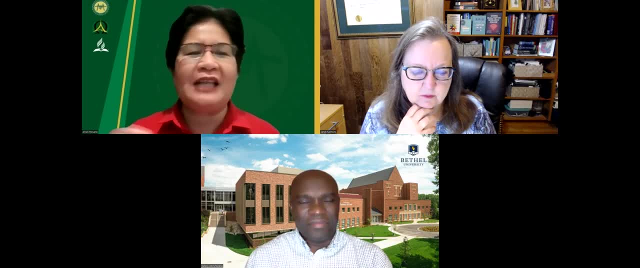 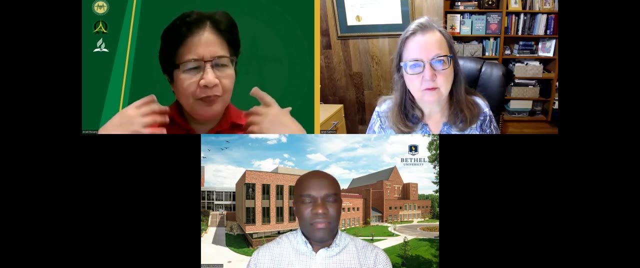 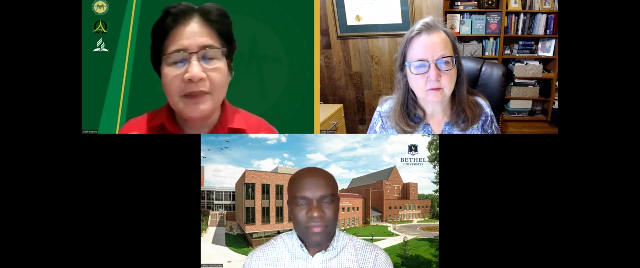 has there been a book published on qualitative research in the asian context so far? uh, this is the only one as far as we know. so this is beneficial because, uh, people, i mean we, we speak in ways i'm talking about myself, i'm an asian, i speak in ways that. 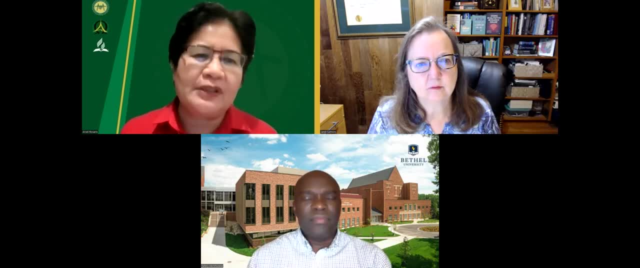 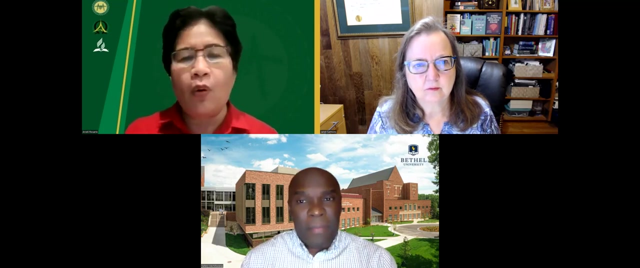 are easy for other asians to understand: mm-hmm, the way we express ourselves, our thinking patterns, mm-hmm, that's, that's. uh. i tried to communicate how how asians communicate, being an asian researcher, asian myself, so it is easy and i've tried to show. 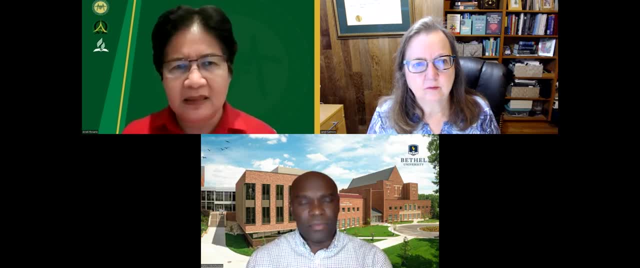 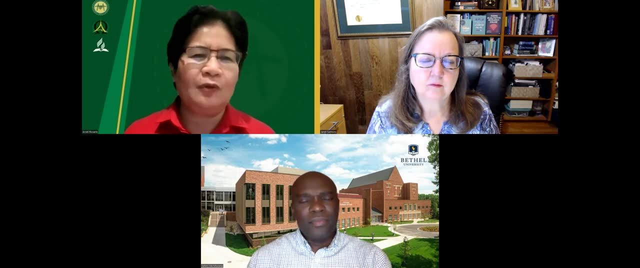 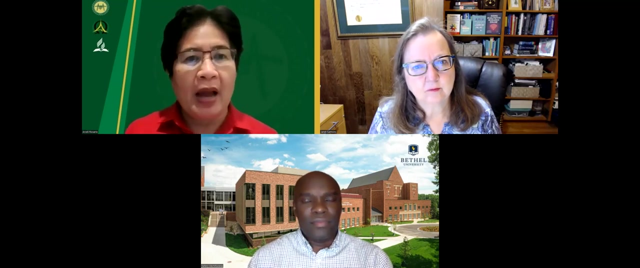 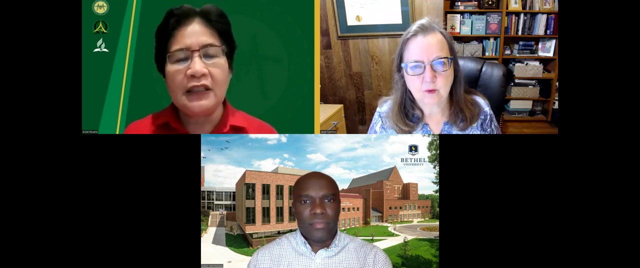 show my works to other asians, how easy it is, and they said, oh, this is easy. uh, we haven't uh thought that qualitative research, which we consider difficult, can be presented in this way. and another one is because, um, It is inspiring for Asians to see that we cited Asian works of Asian authors in qualitative research and also studies in qualitative research conducted in Asia. 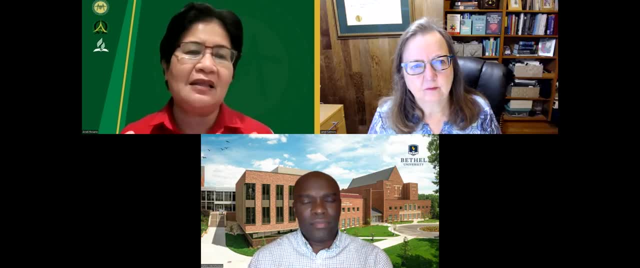 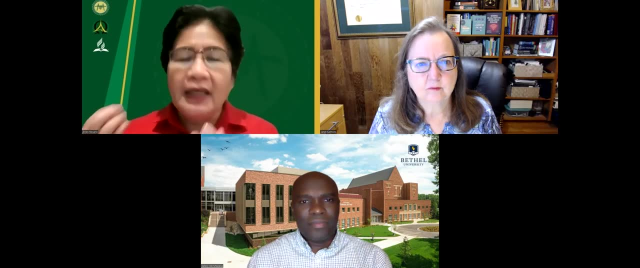 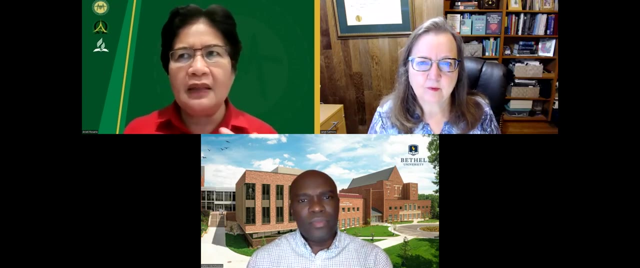 I think that is what makes it appealing. They see, they read findings of research studies done in their context, So that is what makes it appealing to readers. It's like: oh so this is done in my country because I think we were intentional and we instructed our authors. 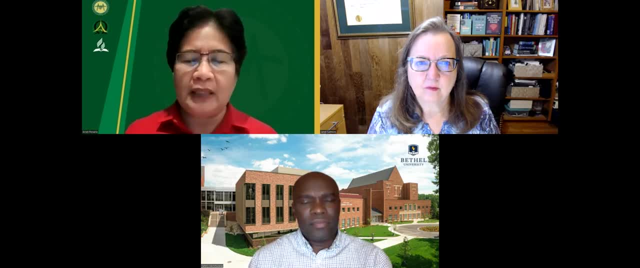 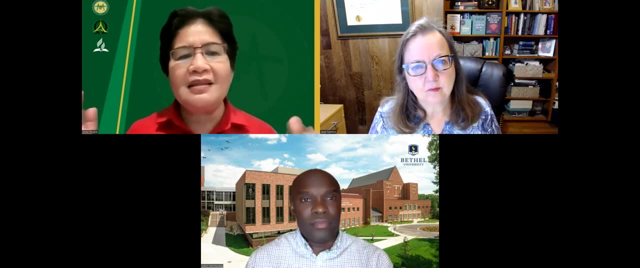 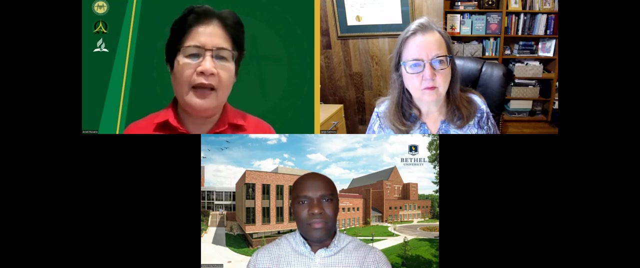 For example, I wrote a chapter on qualitative research and my co-authors and I tried to do, we did like a meta synthesis. We gathered studies on photo voice done in Asia and we tried to see so in Malaysia, in Thailand, in Vietnam, in you know, different countries, what studies were done using photo voice. 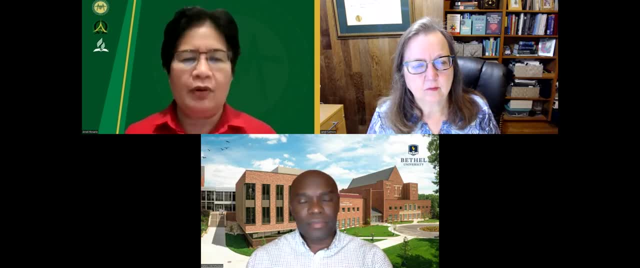 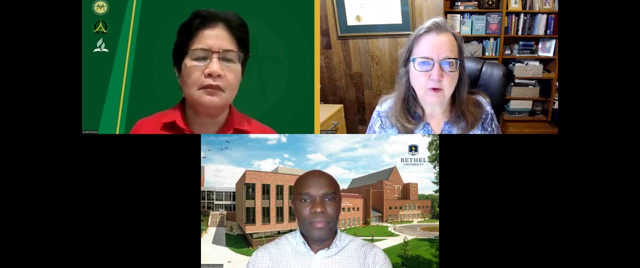 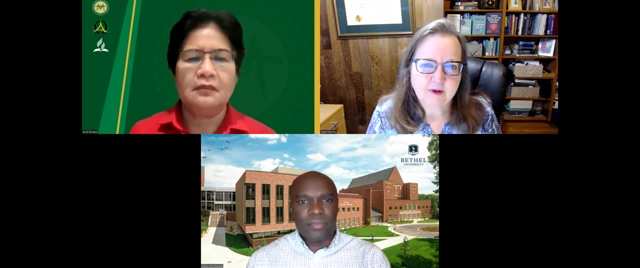 And I believe that one can draw our audience Right because you know it sounds like I mean it's, you know, really an empowering thing to be able to turn to a resource that you know celebrates. you know kind of your own, you know kind of ways of thinking and doing things. 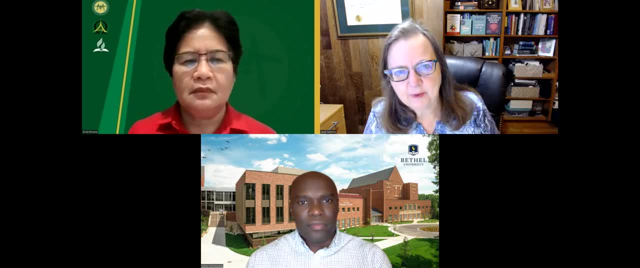 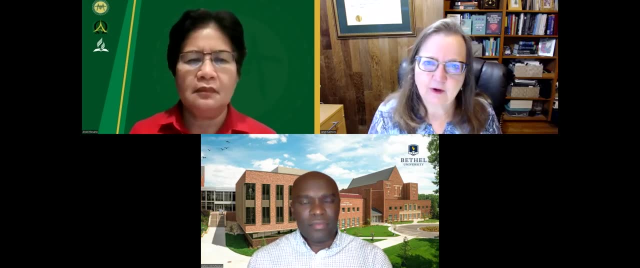 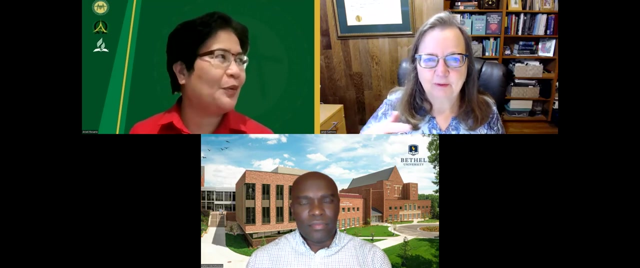 Rather than trying to read something and thinking, well, how does this apply to me? Or how do I translate this into what will work in my setting? And you know, and I very, you know, really want to highlight the point you made about you know, citing studies, you know, so that the people reading this can see- well, it's not only you know. the handbook becomes kind of a roadmap to find, you know, all of this other. 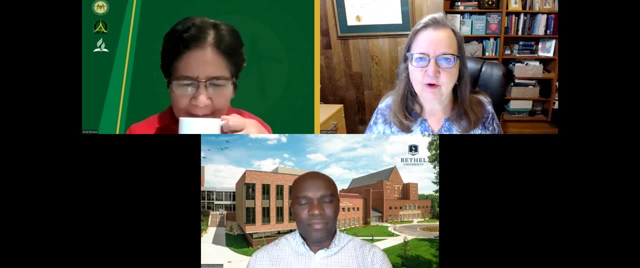 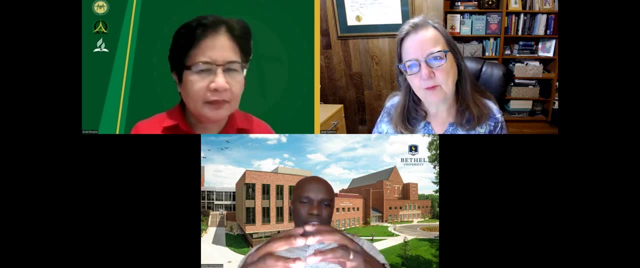 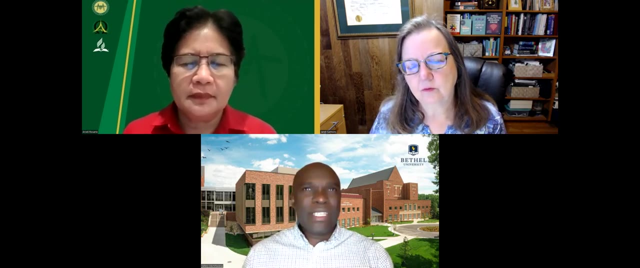 you know body of work that that you know might be of interest, and what would you like to add to that safari? yeah, um, i want to look at it first from, uh, the general perspective, and then from the foreign perspective. uh, from the general perspective, i think this is very, very important because 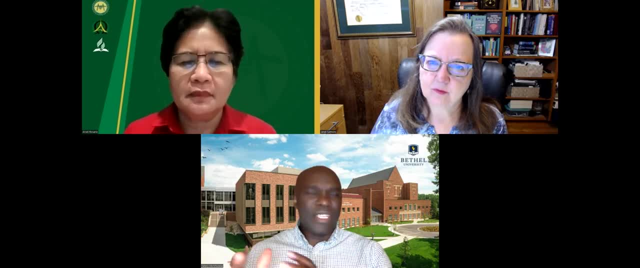 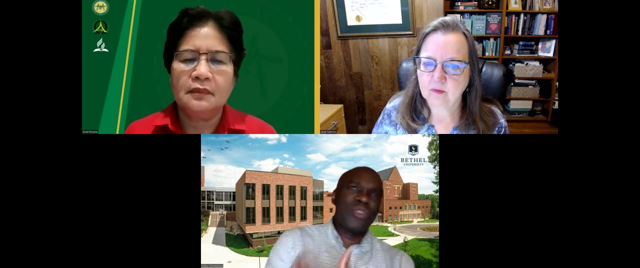 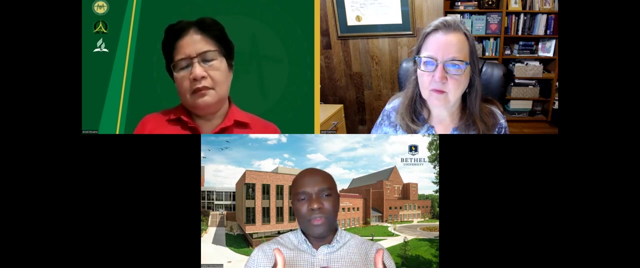 we were able to recruit people from many different asian countries and also people outside of asia who have had experience in asia. i think this helps us to really contextualize qualitative research in a very particular way. um a number of chapters, we compound the authors in such a way that will have an asian and a foreigner, so that 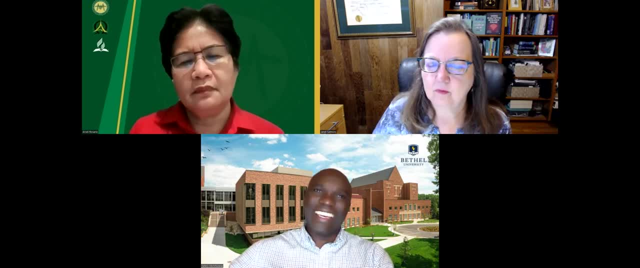 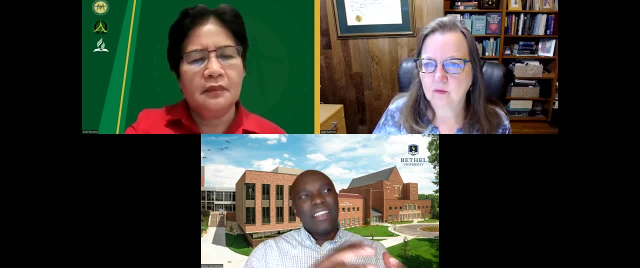 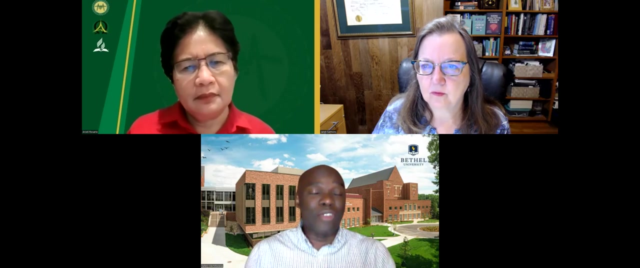 the asian who can bring the original asian perspective in the~~ and the one who is from outside of the Asian context could help fill in the gaps where things are needed for the foreigners From the foreign perspective. as a researcher who was not born in Asia, 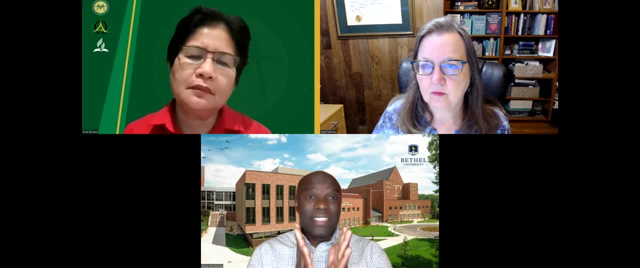 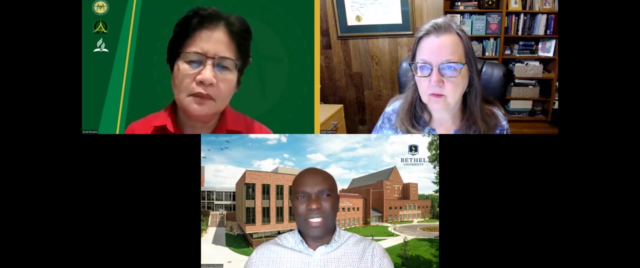 or raised in Asia. I think this is really, really, really, really a great resource, because even myself, as I was working on it, I co-authored some chapters, for example, how to establish a strong relationship between a researcher and a participant in the Asian context. 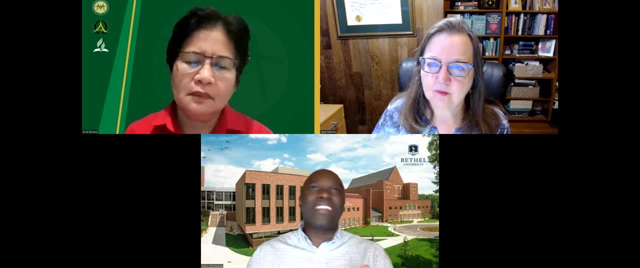 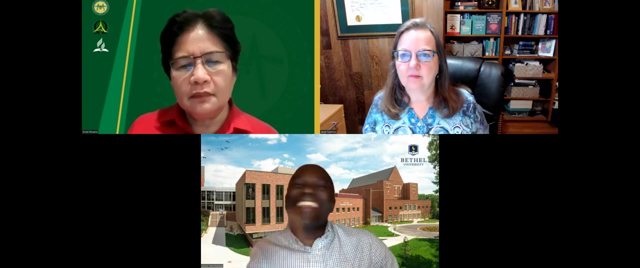 I was one of the authors, Arsely was one of the authors of that chapter, and another one was from Russia and another one was also from the Philippines, And it was interesting, as we're going through this chapter, certain things that I never, ever imagined. 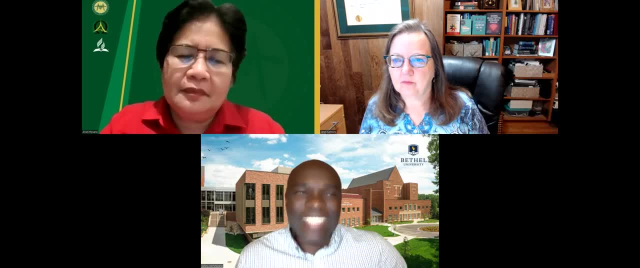 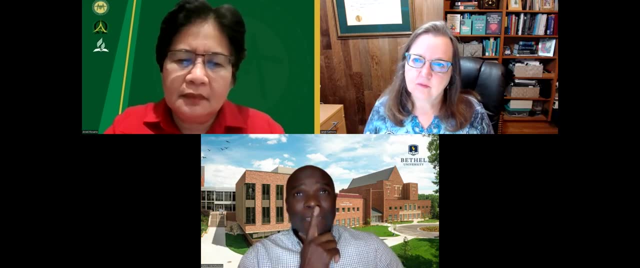 at all that we need to keep in mind, Things that for me, who is a foreigner, wouldn't have thought about. There's another chapter, written by a contributor from Thailand- two contributors from Thailand- where it is all about the culture. 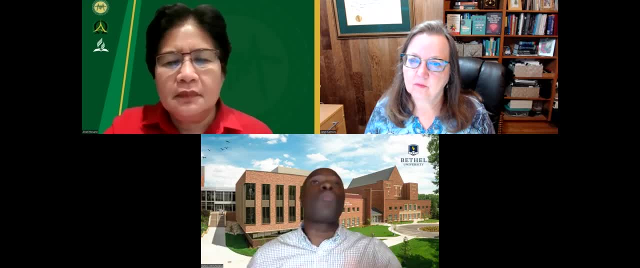 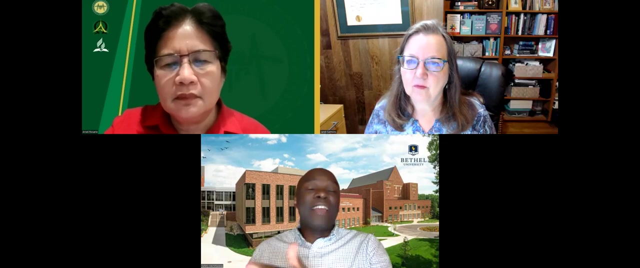 the big culture and where it comes from and what it means for a qualitative researcher. And, of course, for each chapter that we had, we made sure we required all the contributors to show: okay, what are the concepts? What do we need to know in the Asian context? 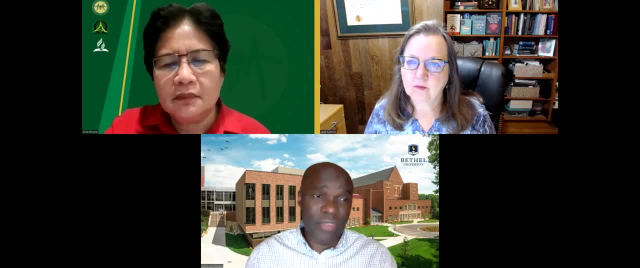 And because we had people who were coming from different parts of Asia or had worked in different parts of Asia, they were bringing in different perspectives of Asia to their culture. It's no longer just data collection in general When I'm collecting data in Asia. 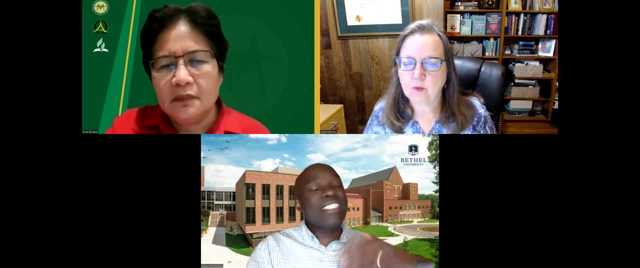 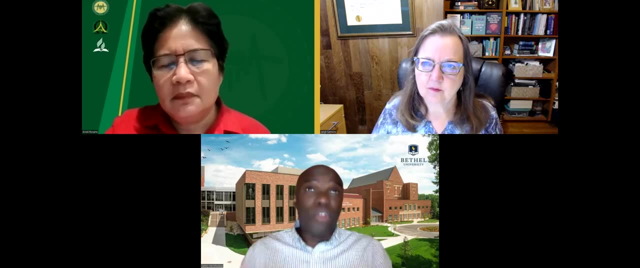 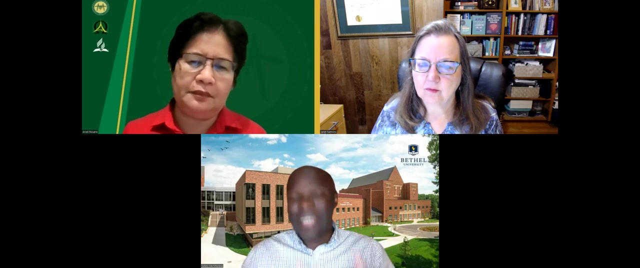 what else should I know in addition to the skills, generic skills, of data collection? And so I think it's. it's a great asset for students and researchers faculty who are foreigners in the Asian context, who are conducting research in Asia, because now they are not just going to blindly implement the concepts. 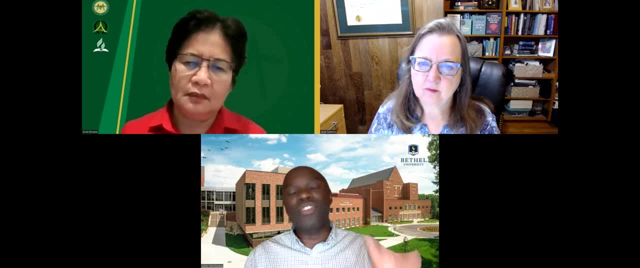 and the skills in the Asian context, but they will really try to contextualize and be aware of the cultural diversity and able to collect trustworthy data, collect data effectively and efficiently here in the US- Just a quick illustration: here in the US. 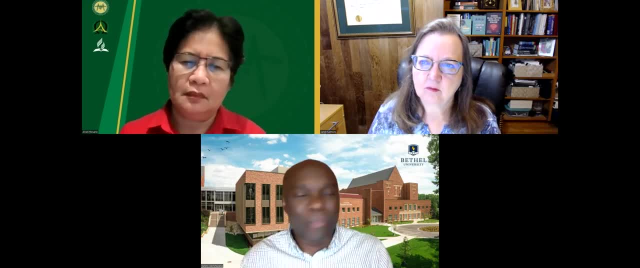 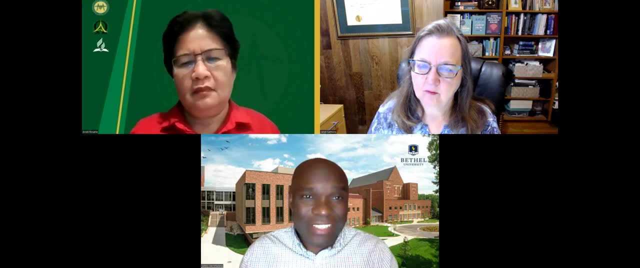 If I'm dealing with a grownup, I don't need to go through another person to ask permission for this person, for an adult, to take to take part in my study. But as you read in some of the chapters, it was amazing when I was reading this. 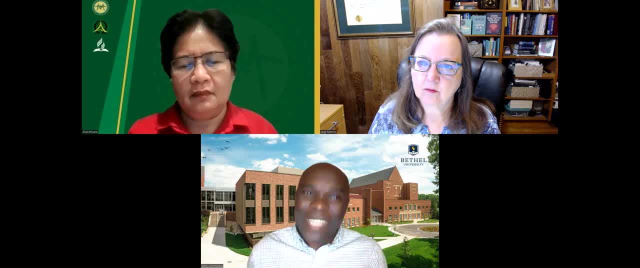 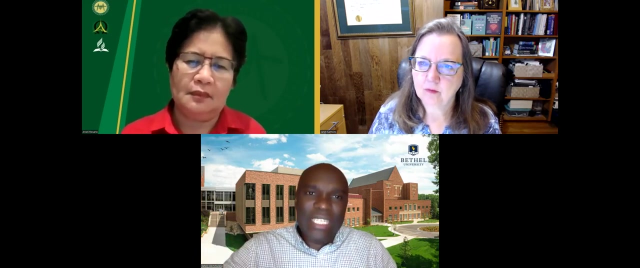 some parts of Asia, and I'm not going to mention which country because one reason I don't remember it. the other reason I want you to read: I want you to read the handbook. You need to convince, you need to ask permission from the elders of the community. 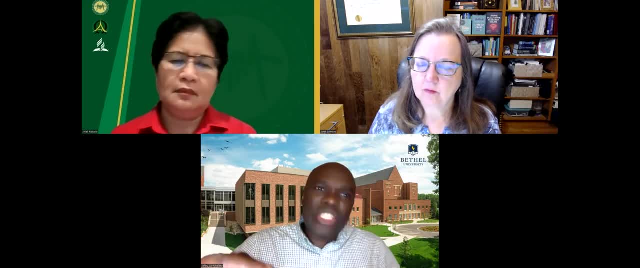 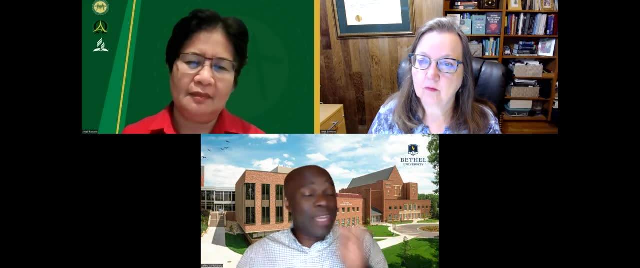 They were the ones to give permission for an adult to participate in the study. I'm not talking about just the gatekeepers. No, I'm not talking about gatekeepers from that perspective, I'm really talking about: did you ask permission? Did he give permission? 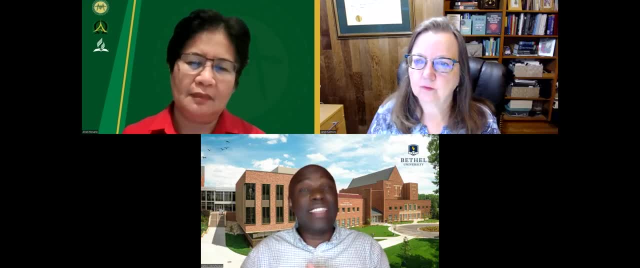 For me to participate, Because if he did not, then that is against our cultural practice. I'm bringing shame to the chief authority. So it's not just about accessing the site. It's about showing respect to the elders and getting their blessing before I can ever participate. 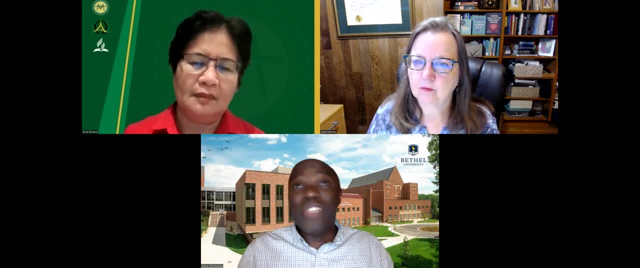 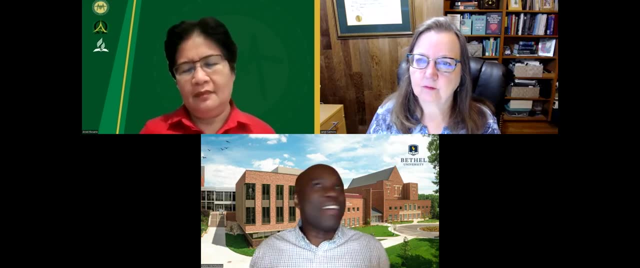 If they don't want, then I don't want to do it, because it is showing that I don't show respect. This is not something you'll find in the West. I mean, you know I'm an adult If I say yes and you have permission to access my university. 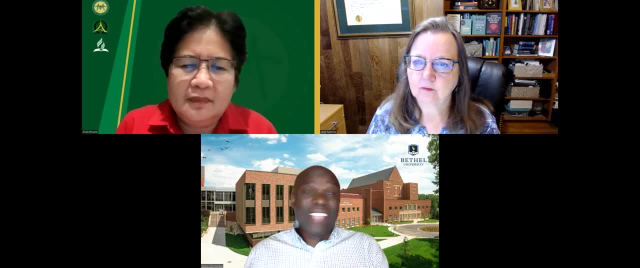 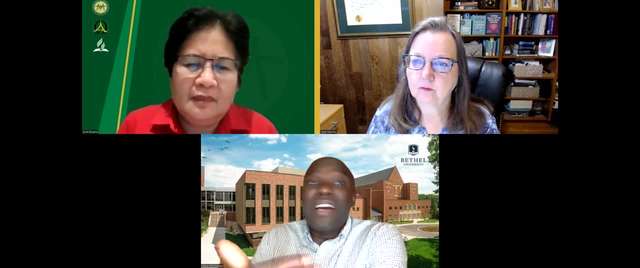 you just have to deal with me. If I say yes, that's it. If I say no, that's it. But in some Asian context that will- I mean in the West- that will count as coercion. If somebody in authority says yes, then you must. 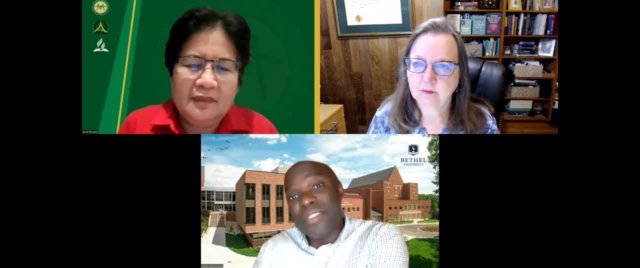 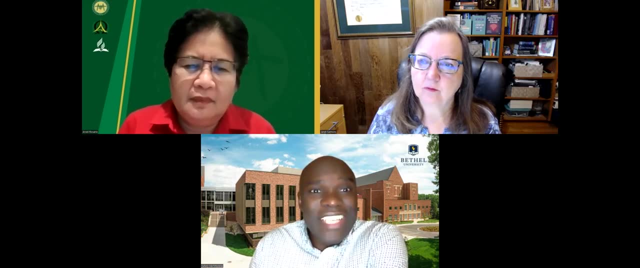 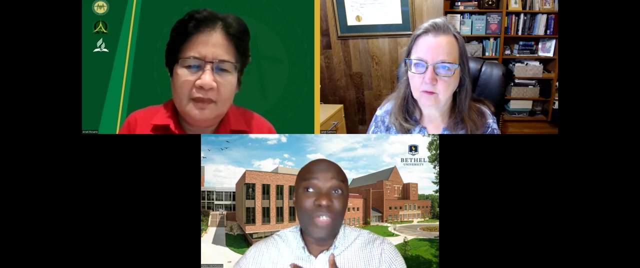 That will be translated as coercion. Right, Because specific settings, some specific settings in Asia, not all over Asia. it's not coercion, It is highly expected, And so, for me, as a foreigner, I need to know about this when I'm going to a specific place. 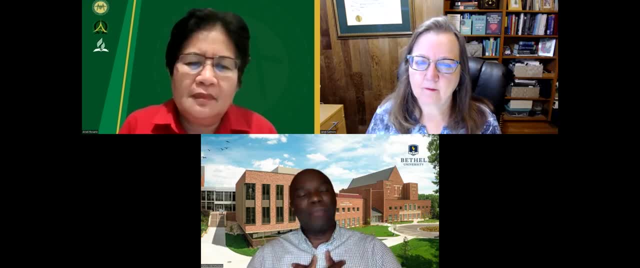 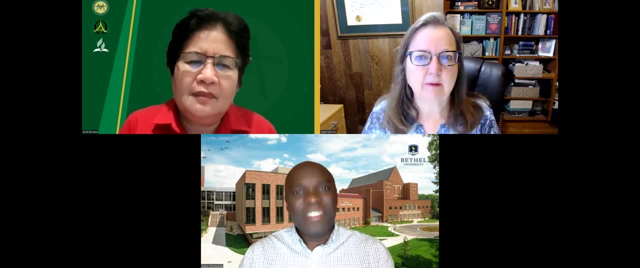 how these things work, so that I will not offend the people who are participating in the study. Right, And it sounds like well. there are a lot of other skills that would go into that, like being able to explain in a very clear way. 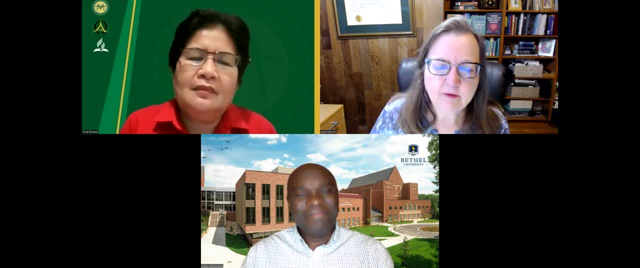 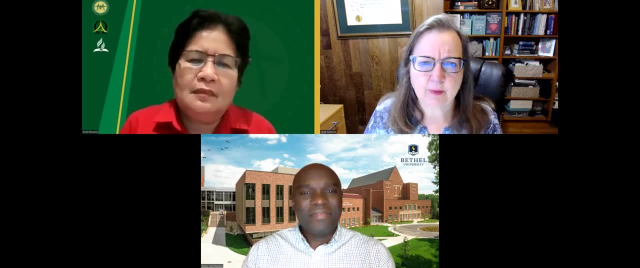 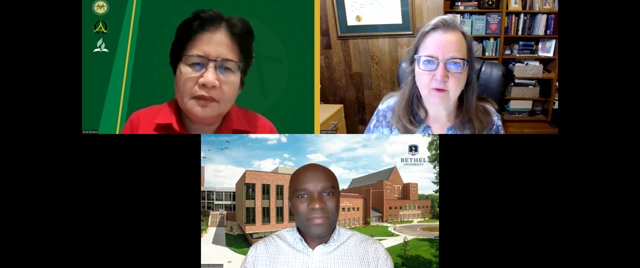 what the research is about and how it will benefit. whatever the topic is that you're studying and being able to explain what you think. that's a whole skill set, And it's also a matter of time. If you're thinking, okay, I'm going to just like fly in. 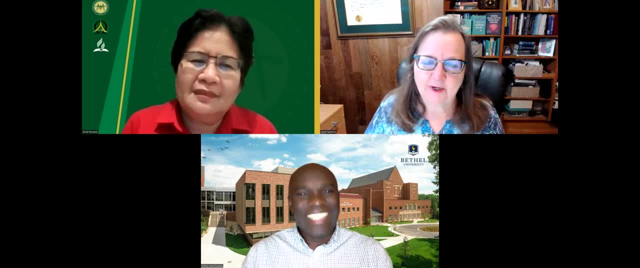 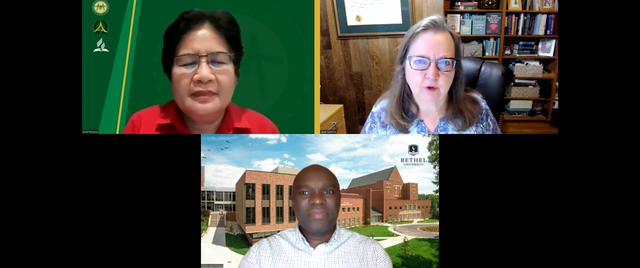 I'm going to do 20 interviews and I'm going to fly home Like no, probably not. So I'm looking forward to introducing this handbook to our Method Space readers And those who have access to the SAGE knowledge database. 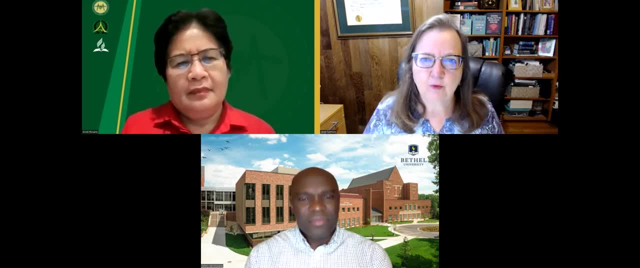 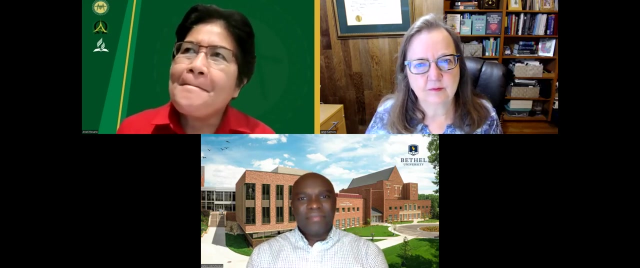 will be able to access the book through there, And you know they can. you know it's a library resource that you can download by chapter and read. So is there anything else that you would like to add? Marcel, do you want to go first? 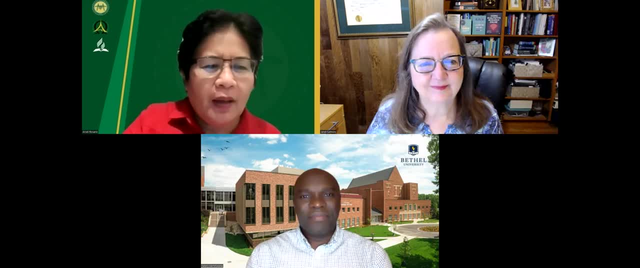 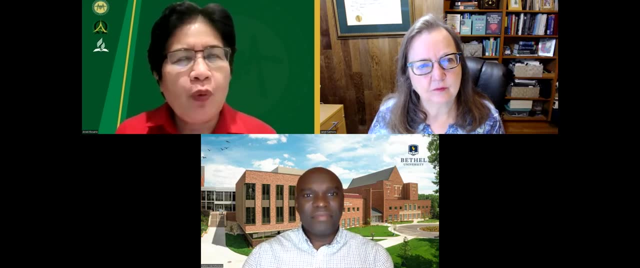 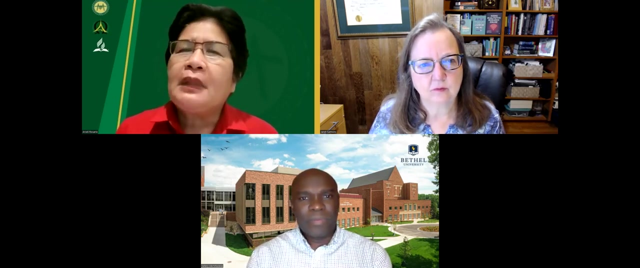 You are muted. Oh, I'm sorry. I think what is interesting about this handbook is we tried to put within the 40 chapters most many, I would say, qualitative research methodologies. For example, case study, photo, voice, Delphi technique. 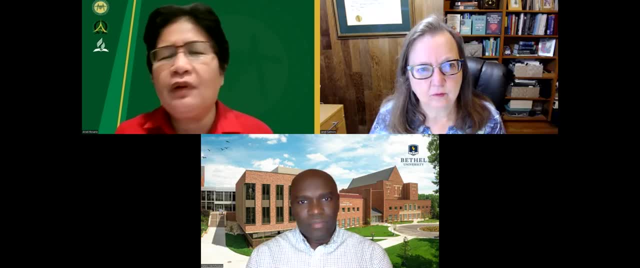 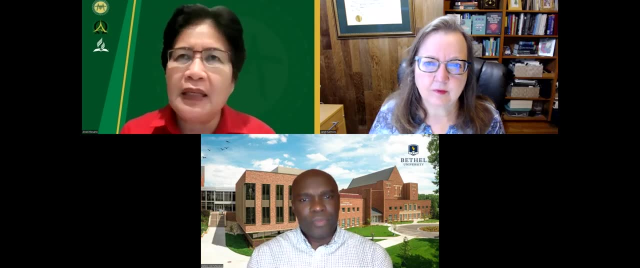 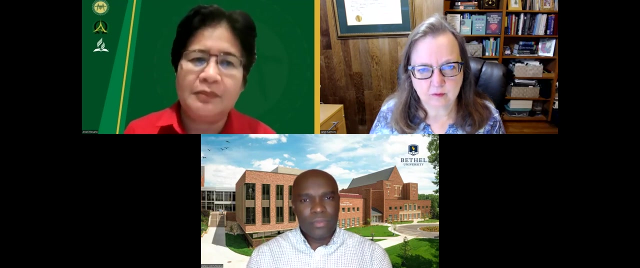 phenomenology, narrative inquiry, ethnography, discourse analysis, So it's like almost complete. So students, those who are doing their thesis and dissertations, and also their faculty, who are advising, they can. they can think of a methodology And there is a high likelihood that they will find this methodology in this handbook. 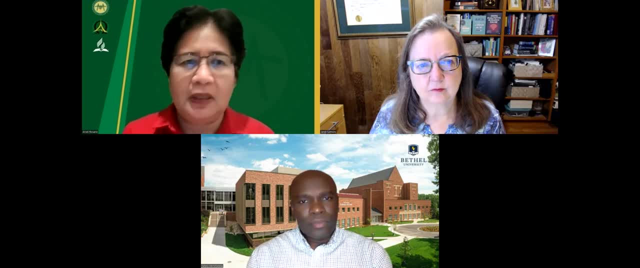 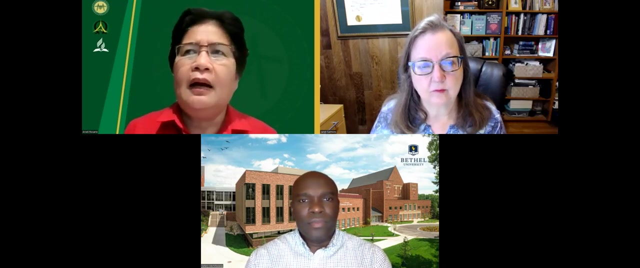 And then we have a section there about data collection And we have tried to address data, different data collection methods and building relationships between the researcher and the participants in also in data analysis frameworks and also how to use the software data, qualitative data analysis software. 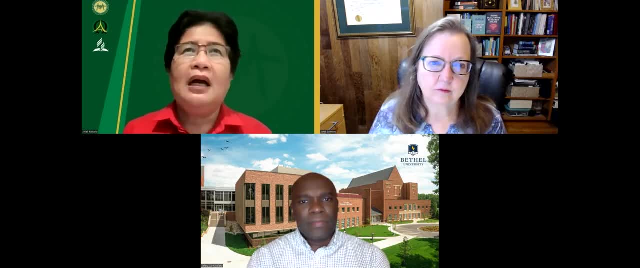 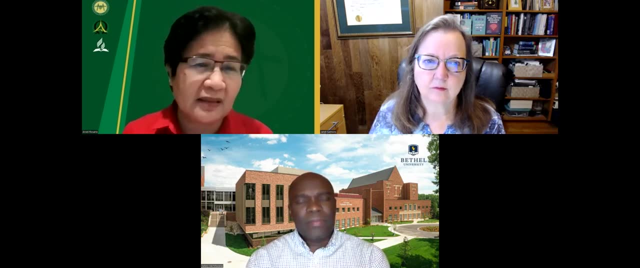 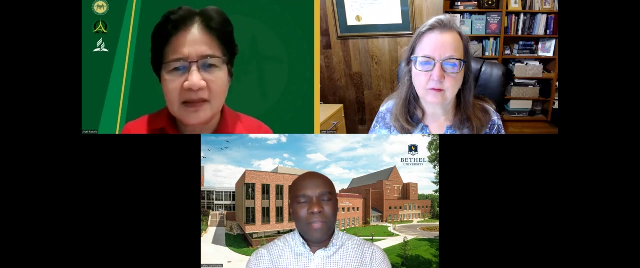 So it is sort of complete from the philosophical foundations of qualitative research, specifically in the Asian context. Until the writing, am I right, Safari? Yes, until publication. And we have addressed their culture, Safari, I think you want to talk about that one culture. 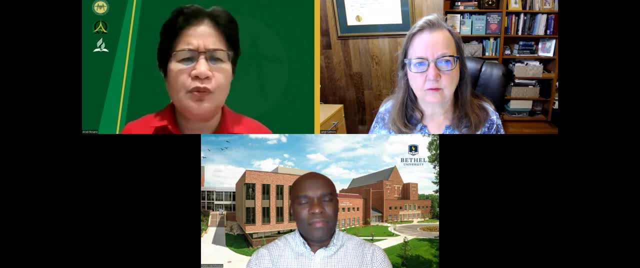 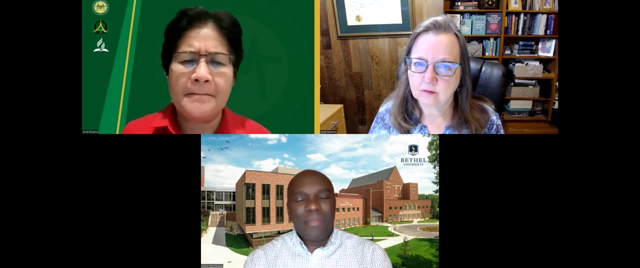 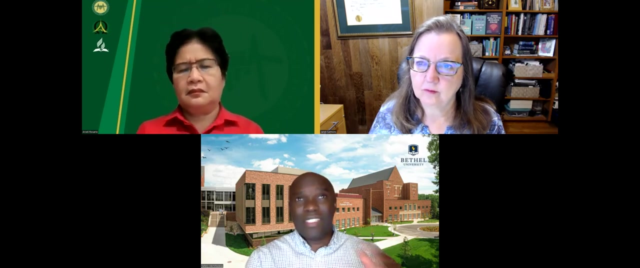 How culture is integrated into or considered in research. Yes, this is a very comprehensive, very comprehensive qualitative research handbook in the Asian context. You get not only the skills, the knowledge of qualitative research which you will find in many other textbooks, but it is contextualized. 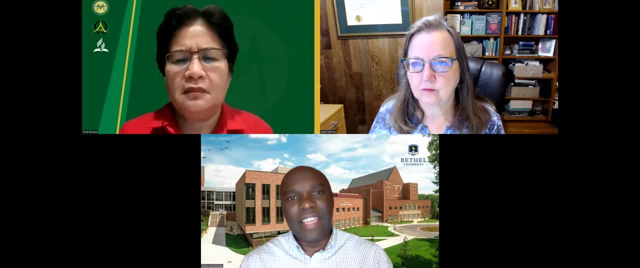 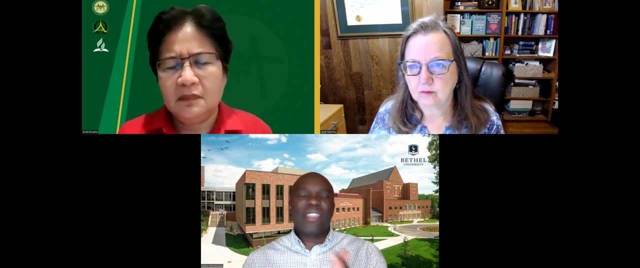 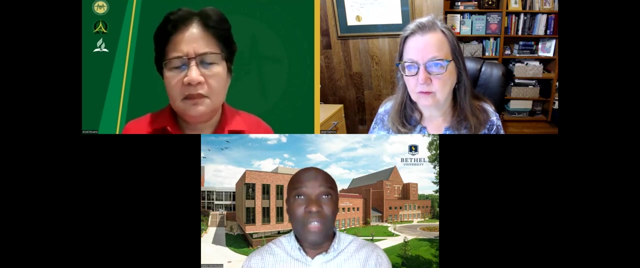 That is the biggest contribution I think that this handbook has. So we talk about a lot of every chapter is contextualized to the Asian context, Asian cultures- And I want to use the plural because there are so many cultures in Asia, although we have some commonalities. 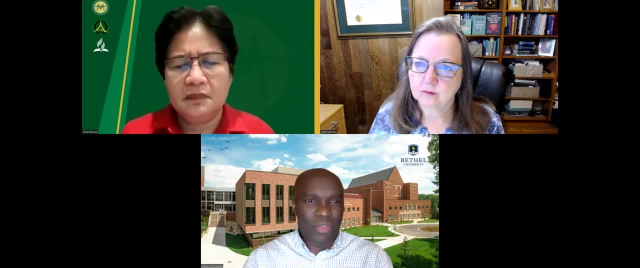 And so anybody who wants to conduct qualitative research in Asia, please do yourself a favor: read this handbook. You may not necessarily read all the chapters, but everything that you want to do- you want to conduct a case study- read the chapter on the case study.